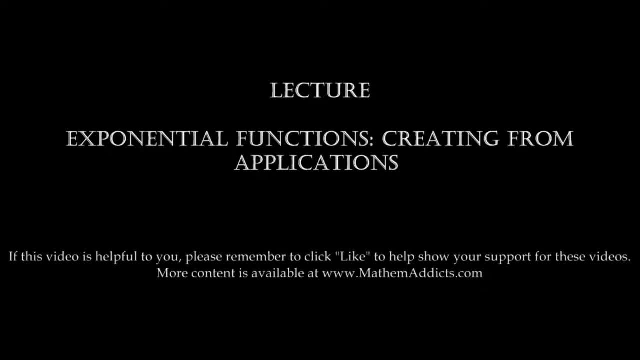 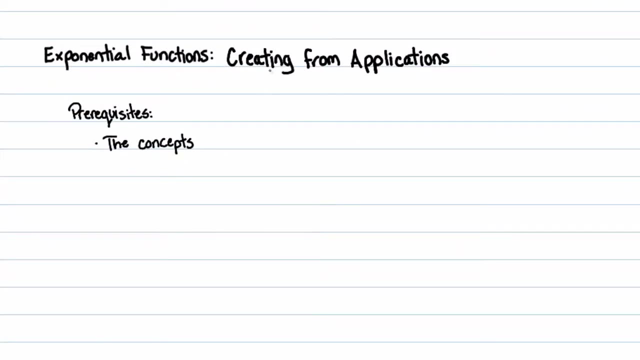 This is the second part in the lecture on exponential functions. In this lecture, we're going to talk about creating exponential functions from application problems or word problems. Really, the only prerequisite you need for this- and the most major prerequisite you'll need- is to watch the concepts video that's supposed to be watched prior to this. 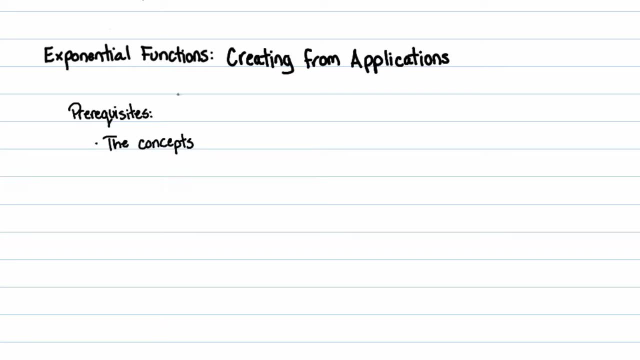 I talk about what an exponential function is. I talk about the parts of an exponential function, all that stuff. I'm only going to briefly review them in this video. I'm not going to introduce them, I'm just going to say: remember this and that's it. 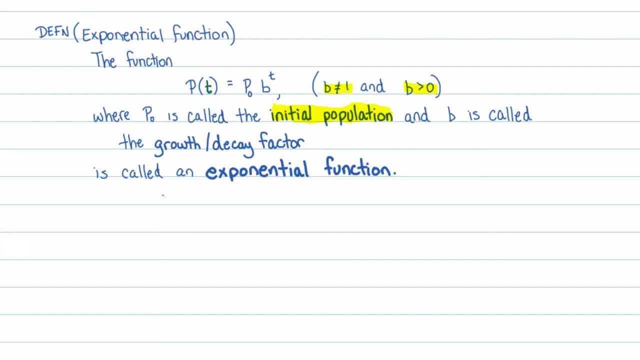 So let's go ahead and define it again. Exponential functions are just functions of the form. p of t is equal to p-naught, b to the t. where b is called the base, p-naught is called the initial population. b is the base of the exponential. 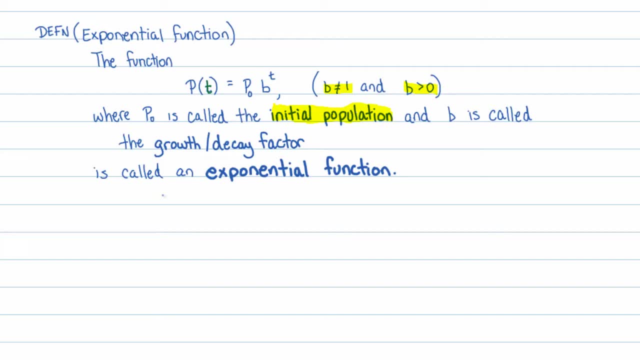 b is the exponential function, but b is also called the growth or decay factor. Let me go ahead and highlight that because I didn't last time, that I in the last video, So I'll go ahead and highlight that here And altogether that is known as an exponential function. 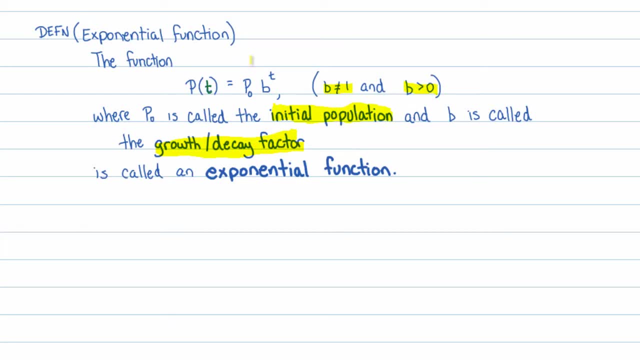 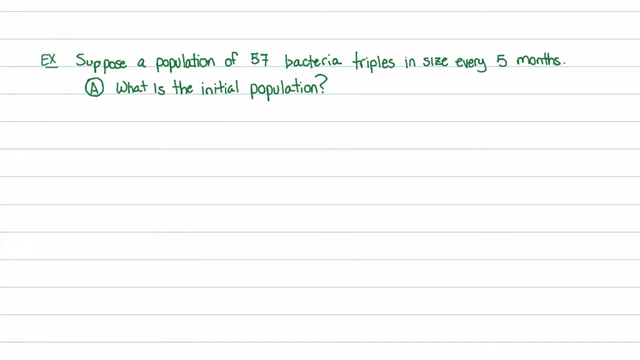 So we have all the parts and pieces that we can talk about, p-naught being the initial and b being the growth or decay factor. So let's take an example here. Suppose that a population of 57 bacteria triples in size. 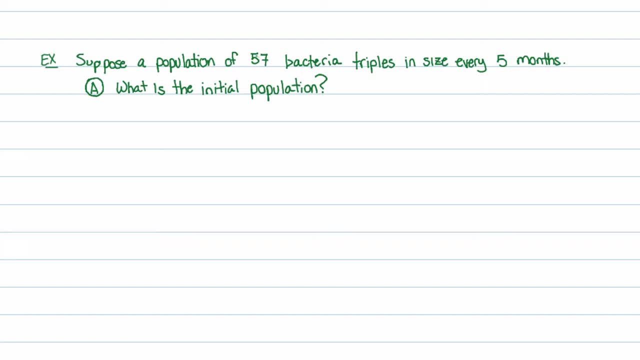 Every five months. This is indicative of exponential behavior, because you are multiplying the population by some number every chunk of time. In this case, it's multiplying by three every five months. When you see that multiplying by a number every so often, it means that you have an exponential growth going on. 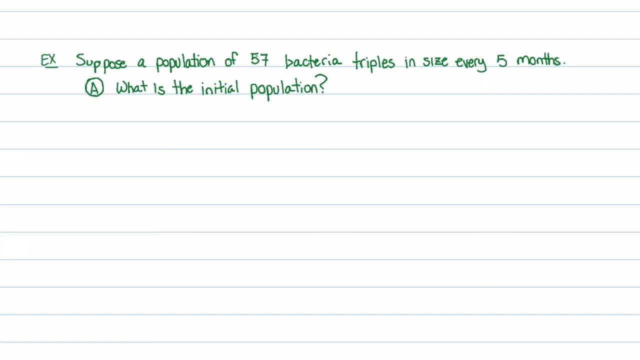 Or possibly An exponential decay. The fact is, the word triple tells us it's going to be growing. So we're tripling every month. It means, you know, every five months means five months from now we'll be three times that size. 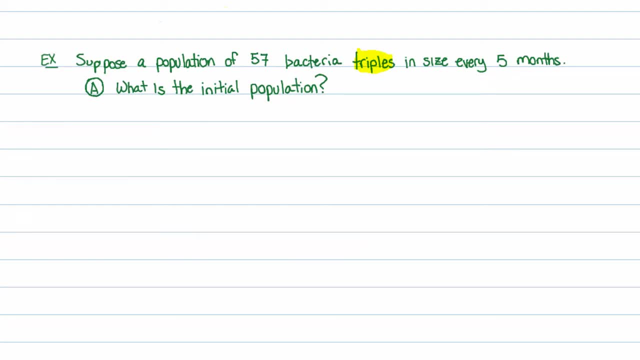 So what is the initial population? I'm taking this in little bits- The initial population which in our formula- and maybe I should write the formula for exponential function first, Maybe I'll write that down below, on the right-hand side, Our formula for an exponential function is p-naught. 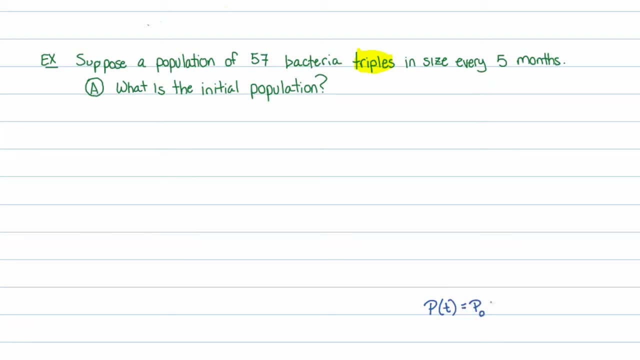 So p-naught of t is equal to p-naught b to the t Again, where p-naught is our initial value, our initial population. Well, the initial population for this problem is 57.. So p-naught here is equal to 57.. 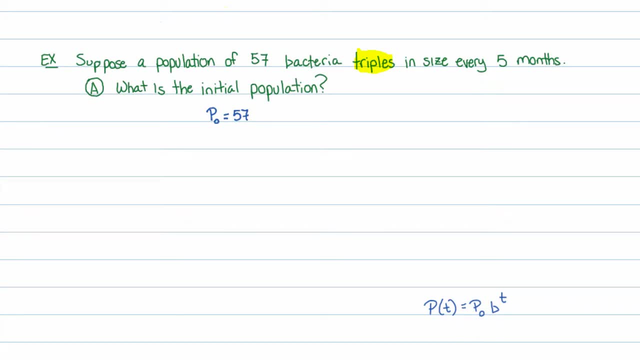 I'm already finding out these unknowns in this problem. Now part b is a little more challenging. What is the monthly? and this is the key word in this problem? You should always pay attention to the wording of the problem. What is the monthly growth factor? 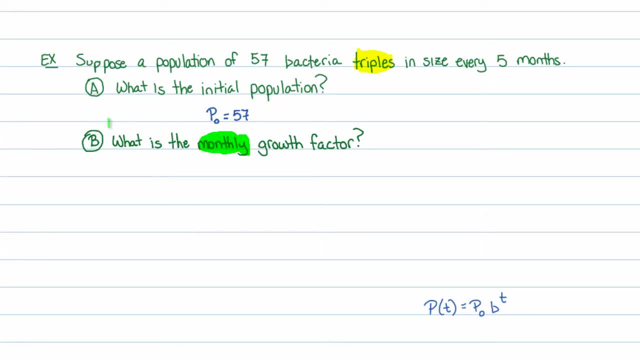 We know that the growth factor is three for every five months, But the monthly growth factor is a little bit different. A great way to kind of approach this problem, to really see what we're going to have to have there, is to write out a table of values. 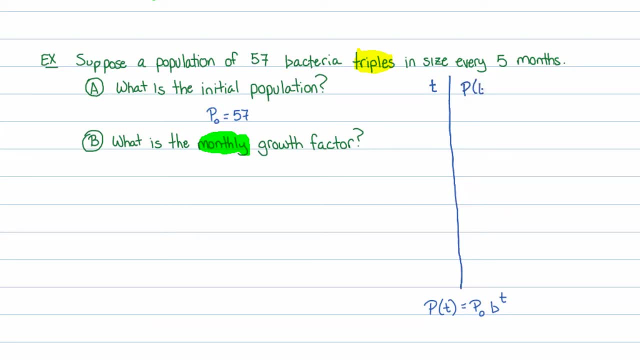 Just to kind of show you the pattern. So I'm going to say time zero, In other words the initial time, Our population of bacteria, what we said, it is 57. And I'm going to leave some spaces in here, not very many. 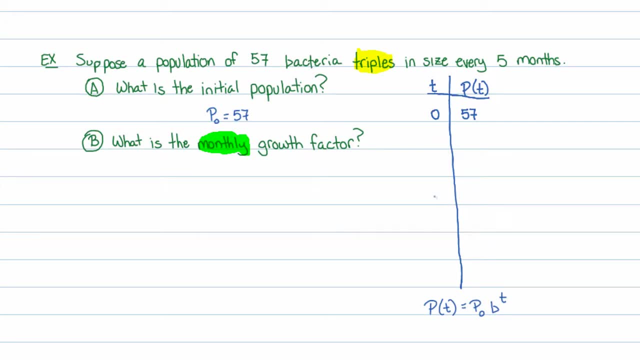 Maybe just a few, like a couple steps or something like that, And down below I'll say five months later. So five months have passed. We know that this population triples every five months, So it's going to be like that. 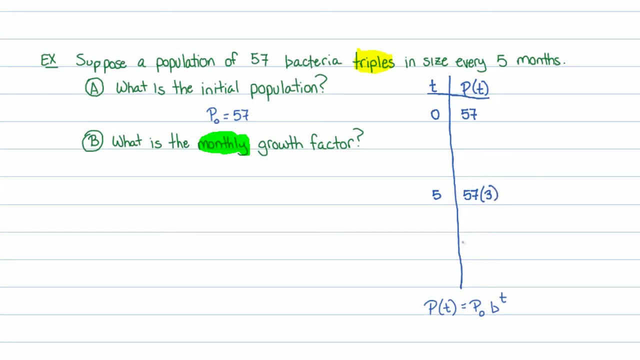 It's going to be like that original population, but three times its size. Another way to write this, by the way, is three to the first power, But more about that later, And then, as time ticks on, ten months down the road, well, the population will be based on the 57 times three. 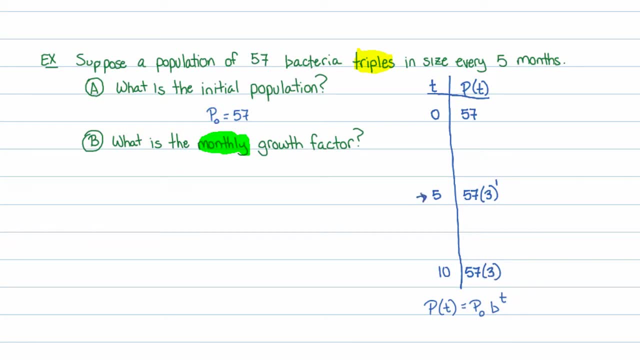 because that's what it was five months prior at the five-month mark, But now, five months after that five-month mark, we're at ten months. we should be multiplying by another, So that's going to be 57 times three, or in other words, 57 times three squared. 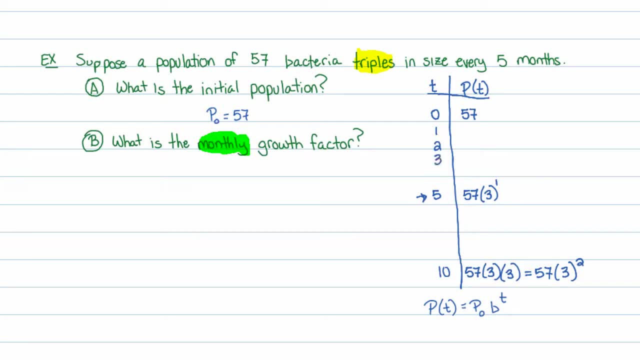 The question is: what about month one, two, three and four? I mean, what's happening in those months? Does it just magically? do we stay at 57 all through those months and then all of a sudden, in month five, we triple immediately? right then, 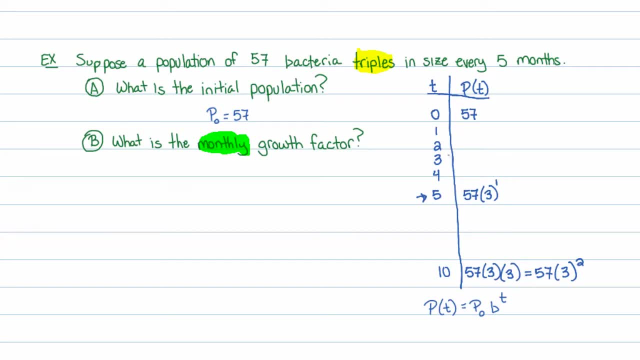 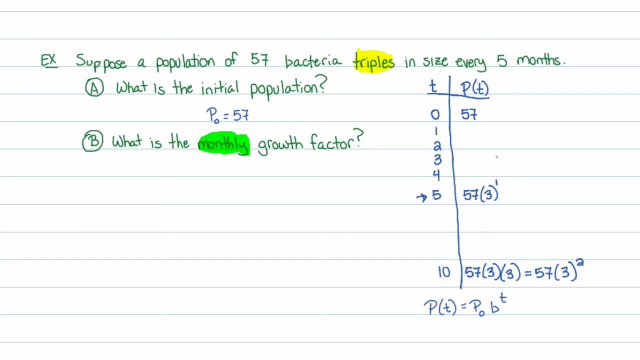 It just becomes triple the size at month five. But it's it takes that long to triple. So let's do a little experiment here. Let's suppose that in month one the population- well it's from, it's based on the 57,. 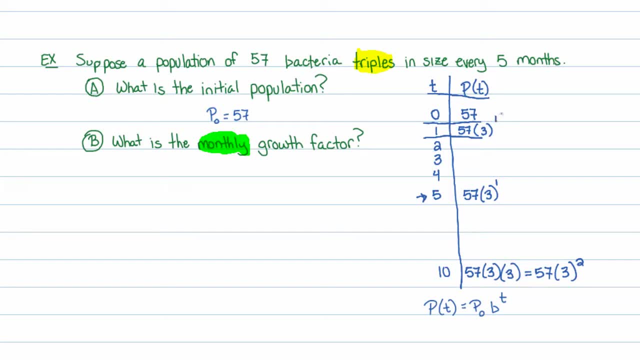 but we're going to multiply this by three, raised to the one-fifth power. And the reason why I chose one-fifth is because I'm one-fifth of the way to a full, I guess a full cycle, full tripling, Because remember. 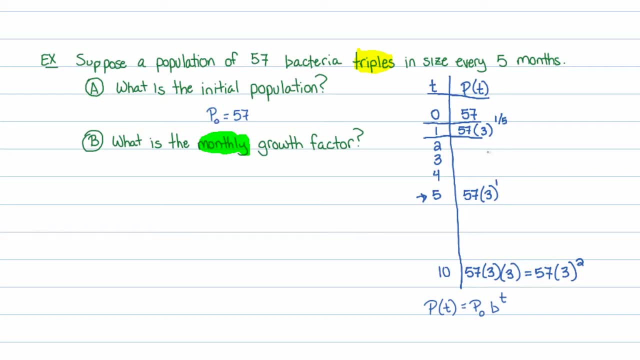 a full tripling occurs every five months. So one month in, I'm only one-fifth of the way in. Now, if I think of every month as being one-fifth of the way to a five-month mark, well then the next step would be 57 times three to the one-fifth. 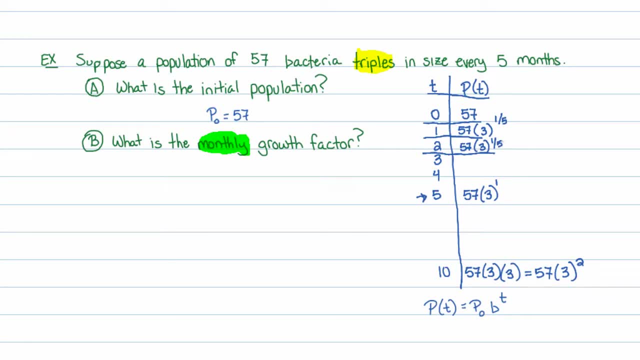 We're going to. it's basically the next step. the second month is going to be the same as the first month, but again times three to the one-fifth power. In other words, I just multiply that last step. 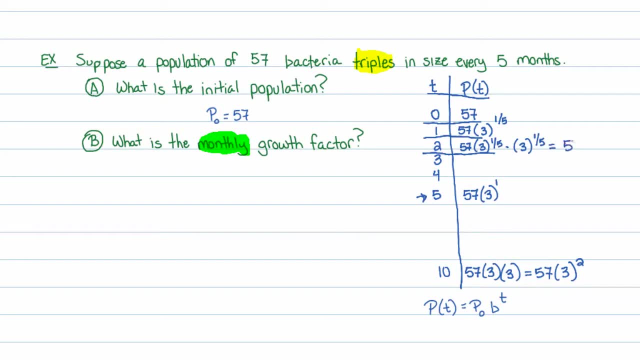 that last value by three to the one-fifth, And if you do the math there, that's 57 times three to the two-fifths. And now you can probably guess the next one will be 57 times three to the three-fifths. 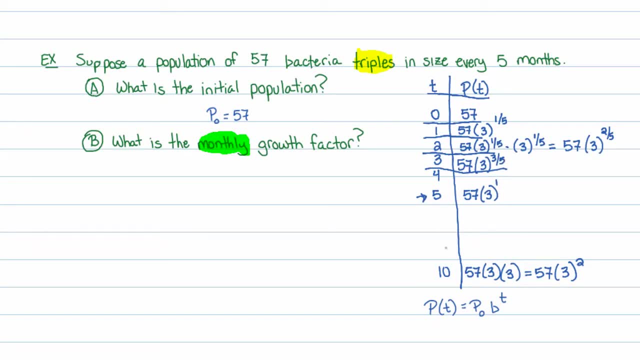 and so on and so forth. It turns out that, in general, if you have a population that doubles, triples, quadruples or whatever every n number of months, then you have, let's say- I'll just put n here- let's say n months later. 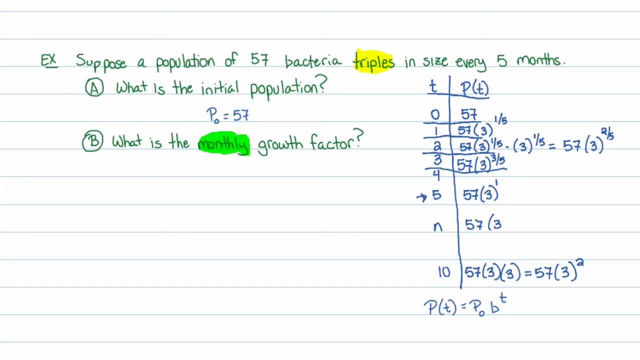 the population's going to be 57 times three to the well n over five, And I'm sorry I said that it's tripling every n months. I should have said let the number of months that pass be n And in this scenario, at that time the population will be 57,. 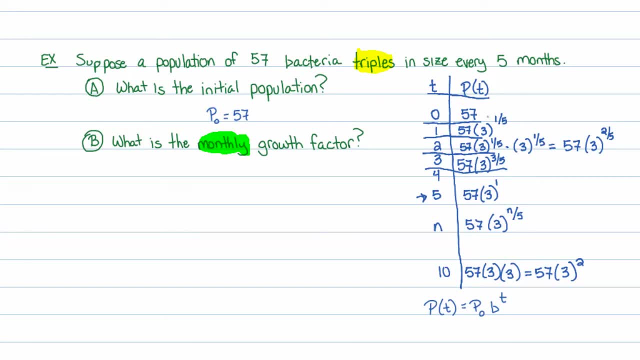 57 times three, raised to the n over five power. just based on this, on this pattern we're developing. But this is asking what the monthly growth factor is. So let's, let's, write the function really quickly. I'm going to go ahead and write it right here. 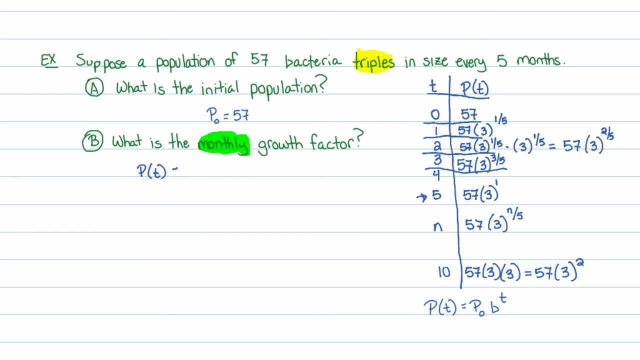 The function now I know is going to be: p of t is equal to 57 times three to the t over five power, because every five months it triples. But my question is that is the growth factor three, Remember in this equation down here: 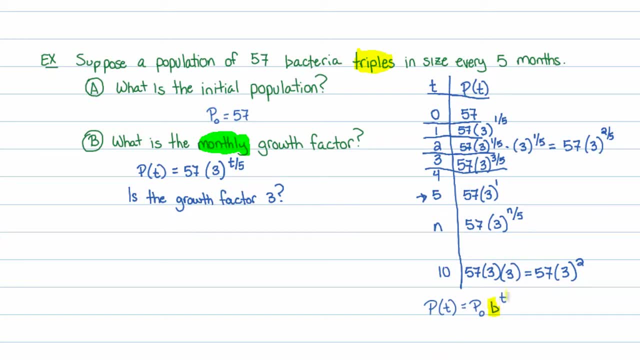 b is considered to be the growth factor, But b has to be raised just to the t, not to the t over five, but just to the t power. So I have to manipulate our exponential function to determine what the growth factor is. So the answer here is no. 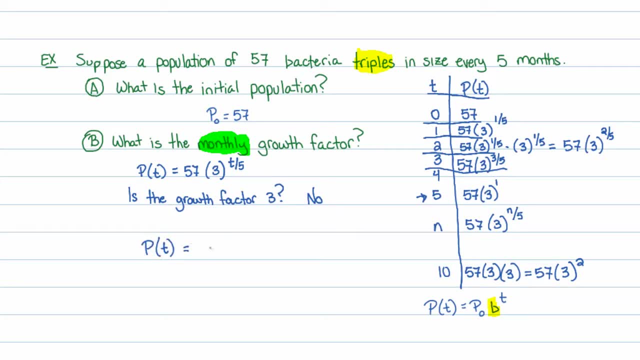 We're going to manipulate this. This can be manipulated to be: p of t is equal to 57 times the quantity something raised to the t power, and that something is three to the one. fifth Powers to powers multiply, so that's still t over five. 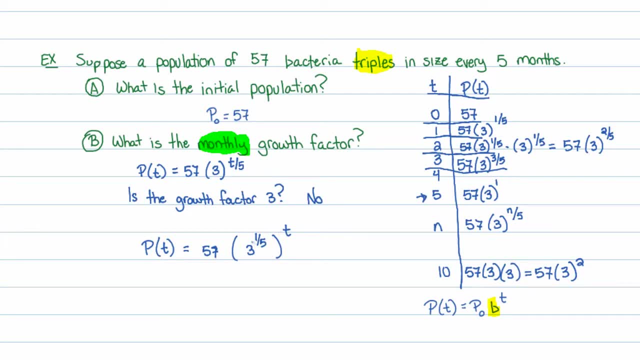 The power is still t over five. I've just brought the one fifth power on the inside. So the growth factor, the monthly growth factor, is three to the one fifth. That tells me by what amount I'm multiplying the population by each month. 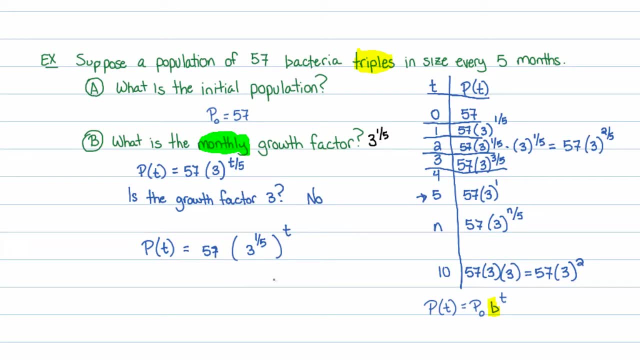 And you could also do this for a daily growth factor if you want to. It just won't be three to the one. fifth, It'll be three to the one over how many ever days there are in five months, So 150.. Let's just say: 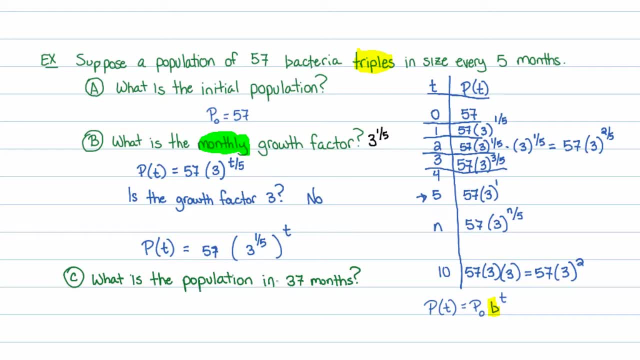 So let's ask a useful question: What's the population of the bacteria in 37 months? Now, remember our exponential function. you can either use this first one or the second one. It doesn't really matter. The second one I just used to answer this question: what's the monthly growth factor? 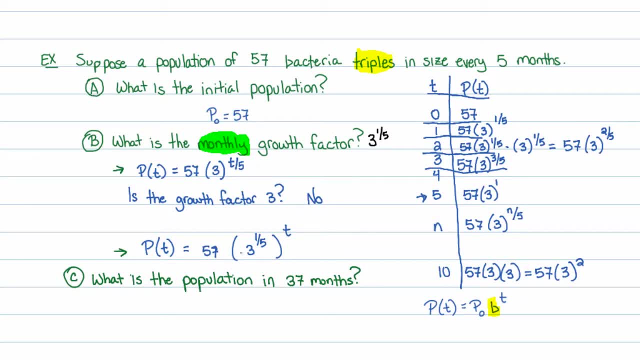 But in reality I tend to use the first one more often than I use the second one for calculations. So what's the population in 37 months? That means let t equal 37, because our time is based on months here, So let t equal 37.. 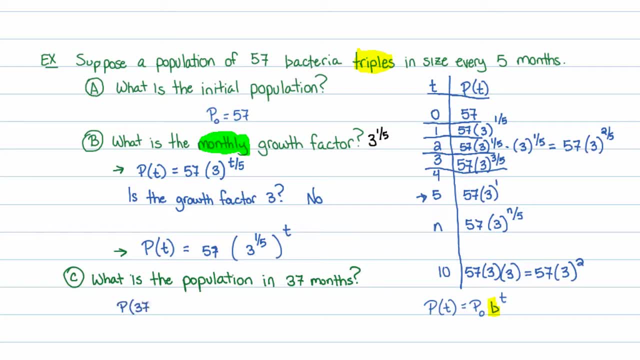 It's really asking what p of 37 is. And again, you see the usefulness of the function notation here, because it allows me to see what I'm plugging in And at the same time, when I get an answer, I can see my output as well. 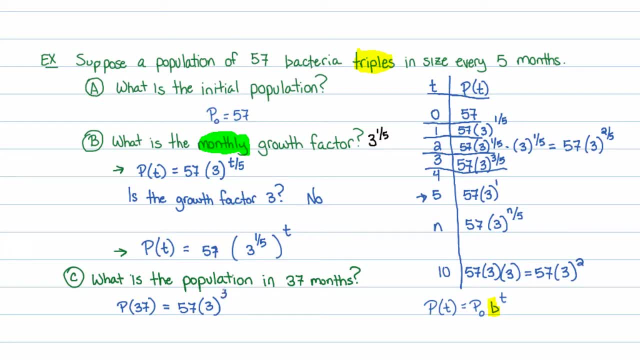 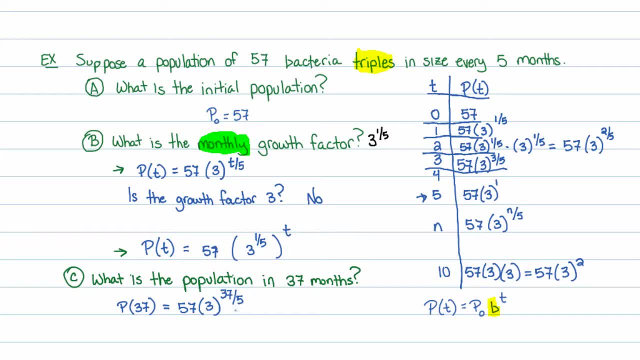 It's a very nice approach to function notation, or the very nice reason the function notation exists. Now I'll tell you right now. this is going to involve a little bit of calculator usage. So let's go ahead and bring up a handy dandy graphic calculator. 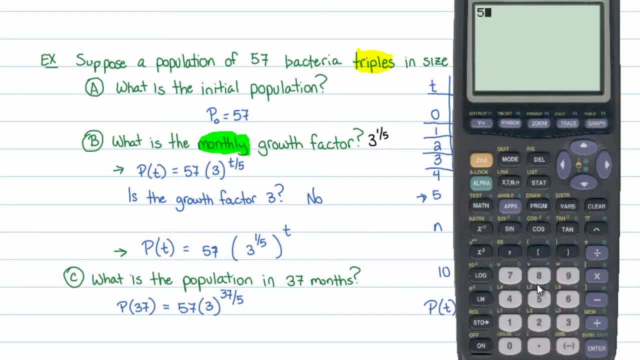 I'll swing that right on over here and I'll type in 57 times. You could put the quantity sign on there. I'm just going to write 3 raised to and then I'll put the parentheses. Remember, when you have math in an exponent, you have to surround it. 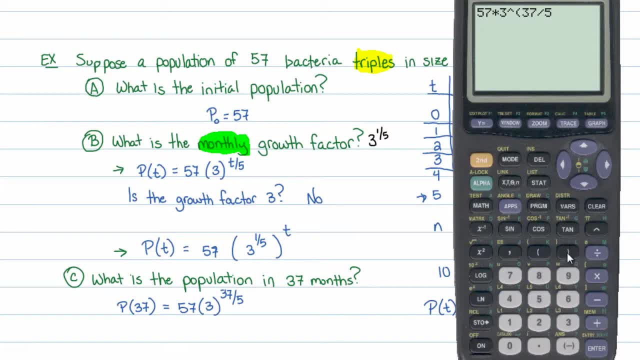 With parentheses. 37 fifths hit enter and I get 193,451 and all rounded to the nearest bacteria, So 452, so roughly equal, or approximately equal, 193,452 bacteria, if you want to do that. So 452, so roughly equal 193,452 bacteria, if you want to do that. 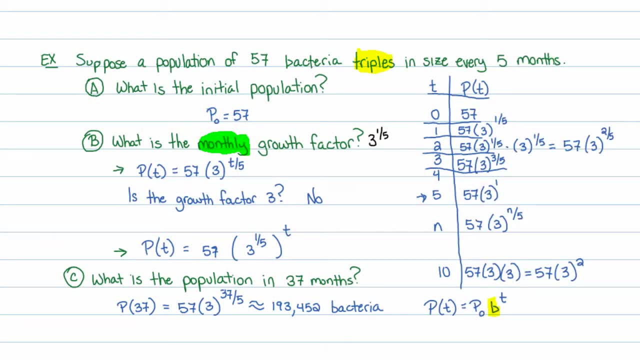 Every single skill I used here is extremely important when dealing with exponential functions. You need to know how to identify the initial population. You need to know how to identify the monthly- or I mean not the monthly, but just whatever the growth factor is, Whether it's daily growth factor, monthly, yearly, whatever you're talking about. 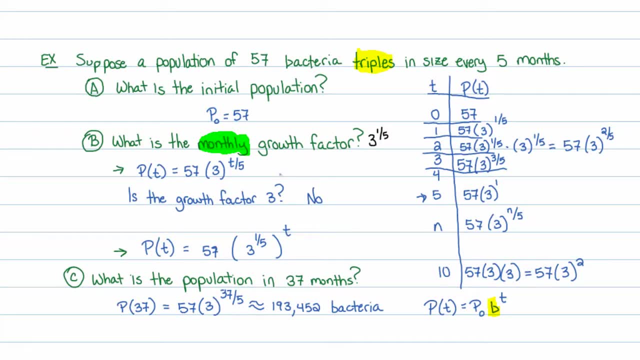 You need to be able to identify the growth factor. It tends to be very important in exponential problems. Finally, you should be able to build a function and evaluate that function. evaluate that function at different input values. Now, honestly, I've been talking growth factors, but I haven't really talked about decay factors. 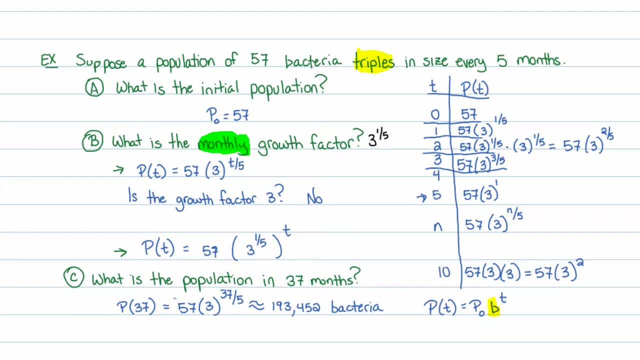 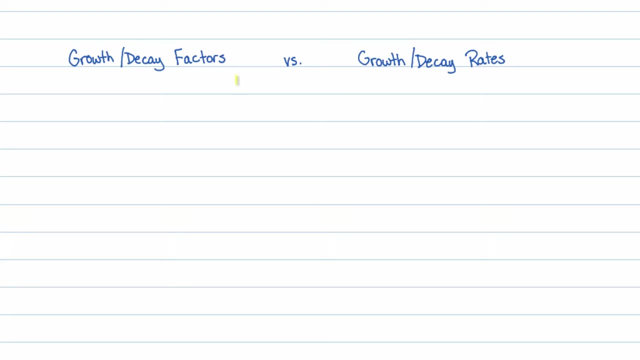 The reason why is that normally, when somebody mentions a decay factor, they usually talk about decay rates. So let's obliterate some confusion with factors and rates right now: Growth and decay factors versus growth and decay rates, and so here's the key words here. 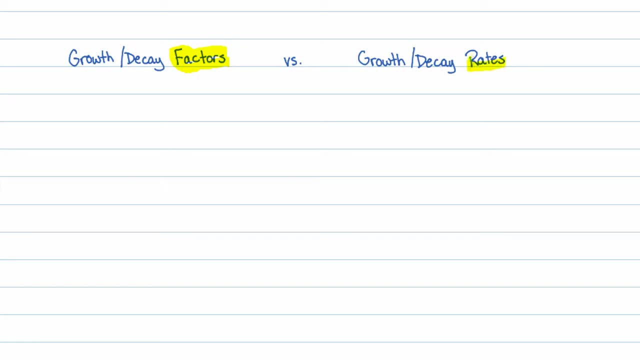 The factors, growth and decay factors versus the growth and decay rates, Two completely different parts of an exponential function. They kind of depend upon one another. They actually do depend upon one another, So they often students get them confused. In an exponential function, p of t is equal to p, naught b to the t. 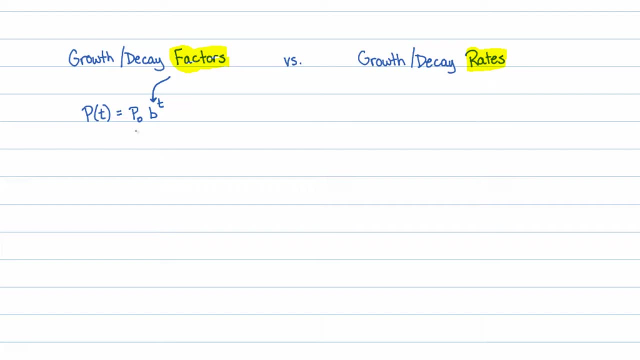 The value of the base of the exponential factor. there is called the growth or decay factor. So b is called the growth or decay factor. However, sometimes you're given an exponential function where b is pretty explicit. It has a. it's still a b really honestly, but some people write it like this: 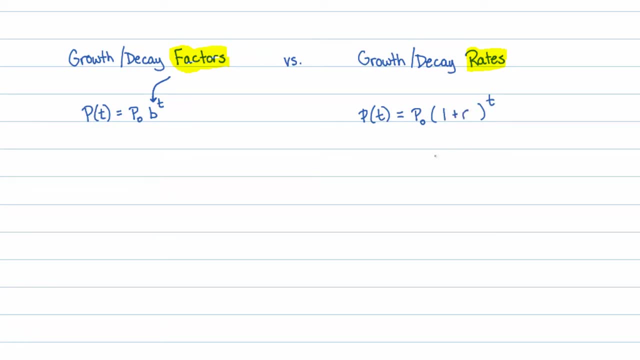 They'll say, oh, one plus r, Okay, Okay, Okay. And when you see this, that little r, one plus r, is the growth or decay factor. That is true, but r itself is called the rate And because we're adding it, that would be known as a growth rate. 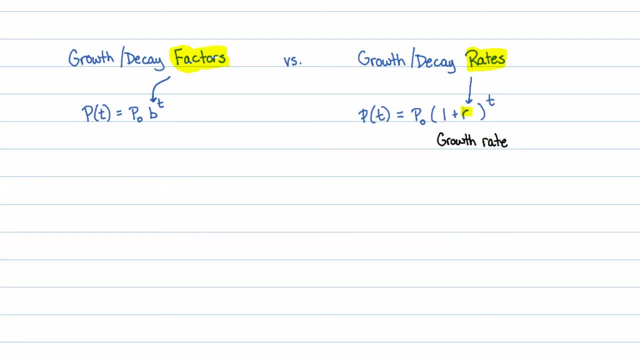 That's if we're adding it. So when you have a plus r, r is just a percentage. so plus 5%, so one plus 5%, That means we're growing by 5%, 5% per year. Along the same lines, if somebody comes along and they hand you a function, an exponential, 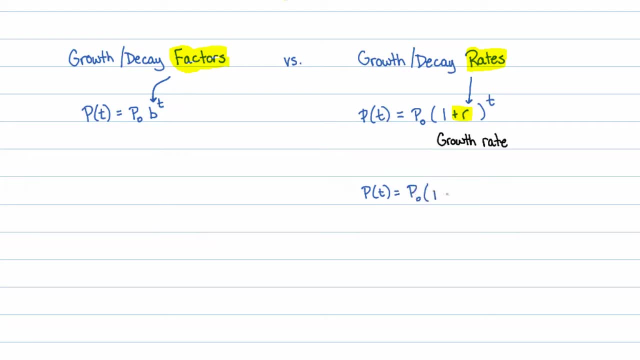 function where you know the unknown is in the exponent, where you have on the inside of your parenthesis, in other words the base, you have one minus r. well, the r there is known as a growth or, I'm sorry, growth, it's known as a decay rate, because you're losing. 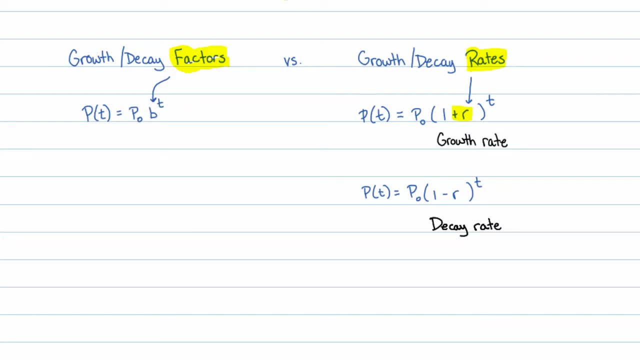 a certain percentage And I'll get more explicit with that in a moment, but I just want to make sure that we get the definitions out there. So when you're adding a percentage, you're growing right. I'm adding 5% per year, or if 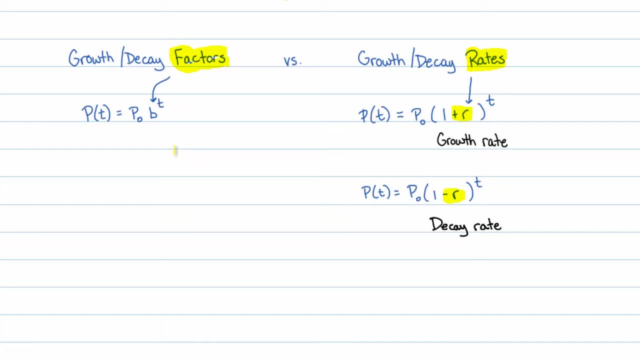 you're losing 7% per year, obviously a population is declining. You know you have a population of the United States. if it's declining by 7% per year, then obviously there's decay rate of 7% per year. So, for example, we've got an example. 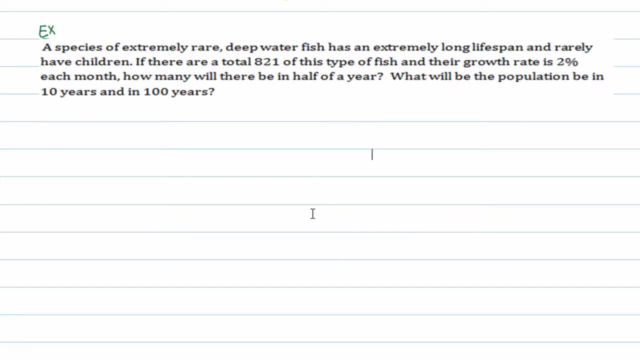 Okay, So, for example, a species of extremely rare deep water fish has an extremely long lifespan and rarely have children, So there's just some fish that just doesn't have a lot of children whatever. If there are a total of 821 of this type of fish in a lake and their growth rate is 2% each month, how many will there be in half a year and what will the population be in 10 years and in 100 years? 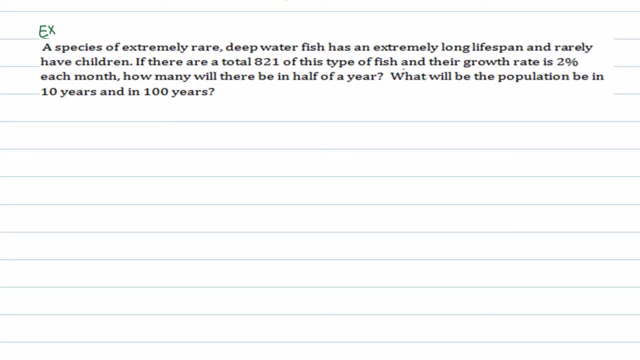 So you have to start identifying parts, because when I tell you you have a growth rate or a growth factor, you know it's exponential. So let me go ahead and highlight that so that we can catch those buzzwords. A buzzword of growth rate: you're growing at 2% per year, or the population is doubling, or anything like that. that means that it's exponential. 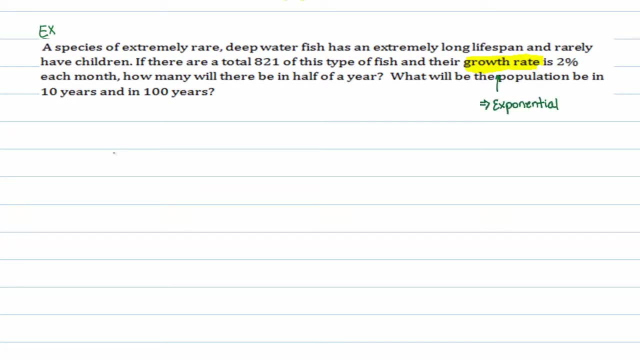 So I'm just going to point an arrow there. So that means we're dealing with the function P of T. It's equal to some initial population times, some base to the T power. So let's try to find the pieces of this. 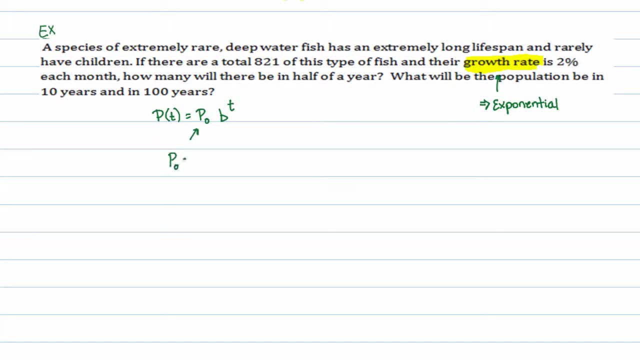 Well, P naught being the initial population, they had to have given us that. I mean, it's not always the case that they have to, but they actually did. The initial population is 821.. They initially had 821.. Now all I need to know is: what is the growth factor? 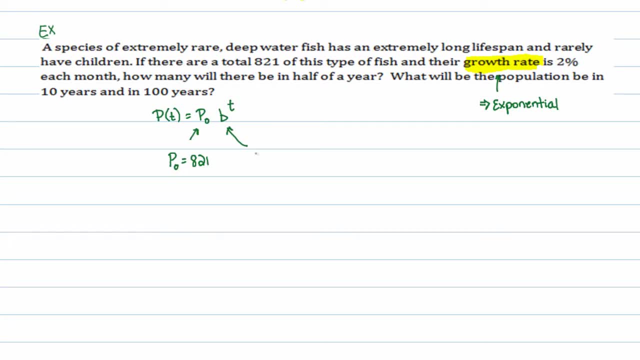 Did they Specifically give me a growth factor like doubling, tripling, quadrupling, or did they give me a rate? If they gave me a rate, then I'm going to have to use 1 plus or minus R in the exchange for B. 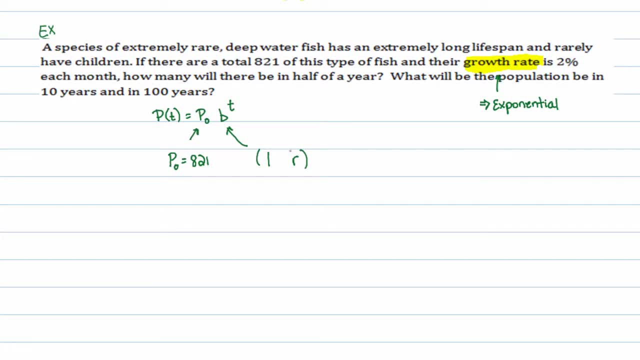 And they gave me a percentage rate of 2 here. so it's going to be, And they told me it's growing, so it's going to be a plus. So 1 plus R, in this case R, the rate is 2%. 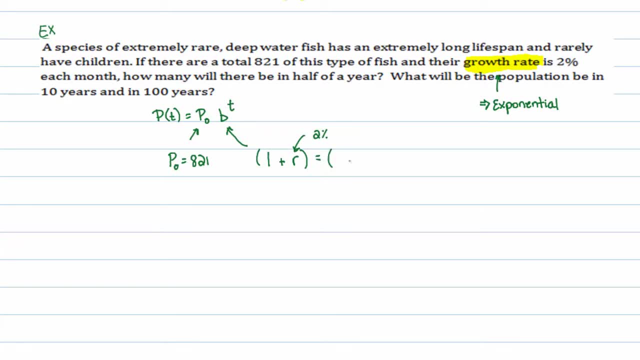 So really, our base for our exponential function is 1 plus 0.02.. That's the decimal form of 2%. So let's go ahead and write that function. P of T is equal to 821 times the base, which is 1 plus 0.02, raised to the T power. 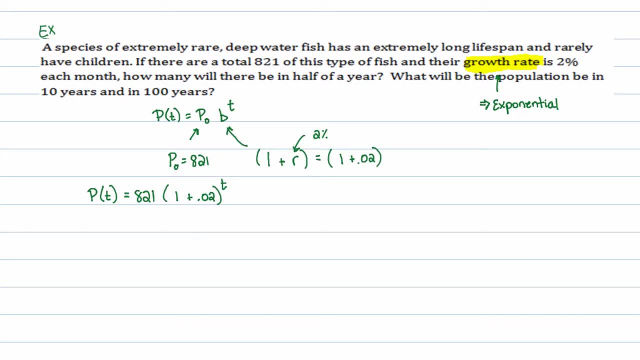 By the way, it's to the T power because it's each month, Not every 7 months. If it was every 7 months, it would be like that: If we were to increase by 2% every 7 months, it would be T over 7.. 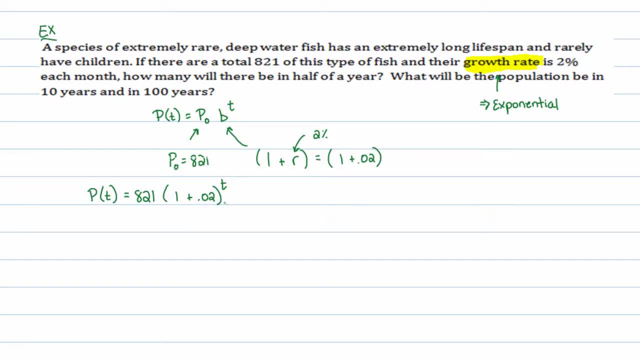 But it's every 1 month, so it's T over 1.. Or in other words, just T, And now you can use this function to do all the rest of the problem. I would probably recommend, or I'd like to recommend, that you rewrite this as P of T is equal to 821 times 1.02.. 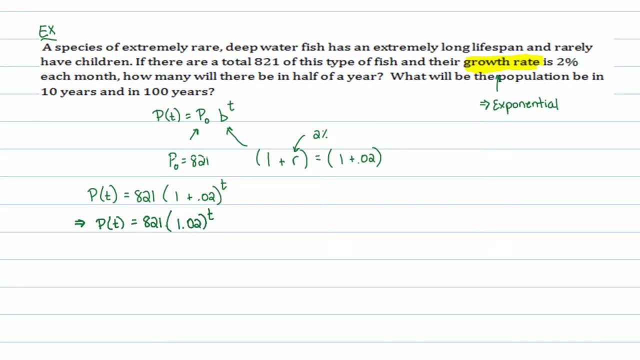 Raised to the T power. I'd like you to also realize that when somebody hands you an exponential function of this form, you should take note. If you have a one point, something inside of as the base of an exponential function, that's somebody telling you the percentage rate that they're growing every year. 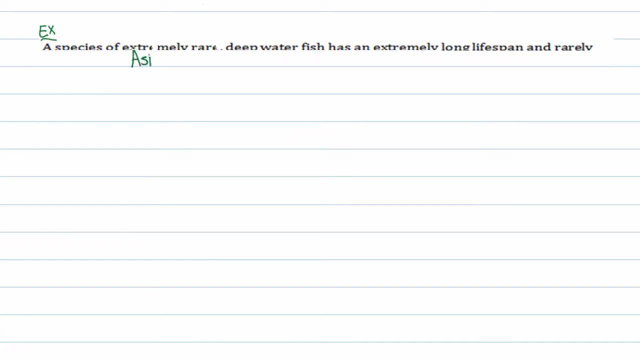 So let me, just as an aside, give you an example of this. Suppose that I said: oh yeah, there's a population And here's the function that determines the population after so many years. Okay, Then you? I've basically told you a ton of information about this population. 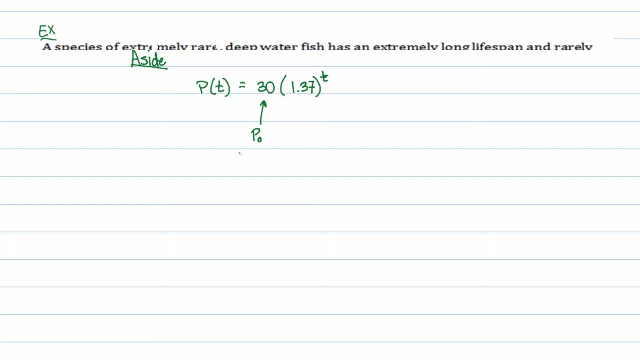 I've told you that the initial population is 30.. So I had 30 of these things originally, And because it's 1.37, which could be written as 1 plus .37 if I wanted to, I already know that it's growing. 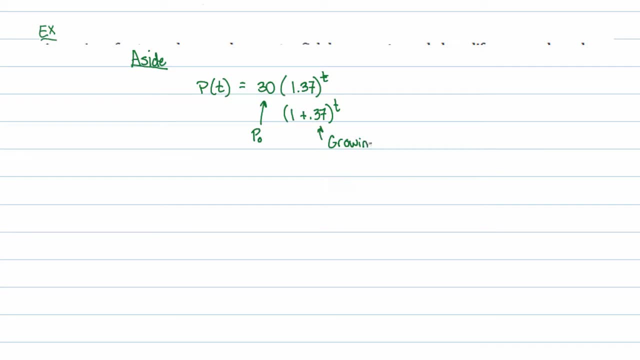 Because it's a plus there- Growing at 37% per year, or per day, or per week, per time, I'll just say per time period. So there's quite a bit you can learn just from the function that you're given. 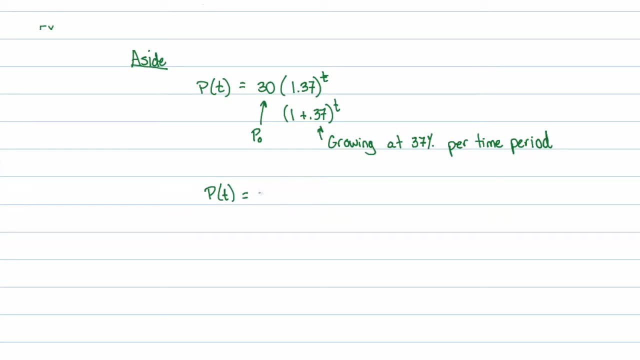 I could do this all day right. I could have. the population of a classroom at the beginning of the semester is 30 students, Or actually? no, that's not true. Normally at the beginning of the semester you have 50 students. in the beginning of the semester, 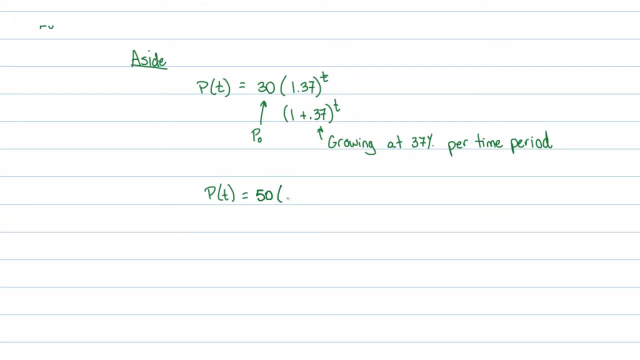 And let's say that this function determines the population of the classroom after a certain number of weeks. Now you might think: well, this is not a 1.95.. So it's not talking about. I can't use what he just told me. 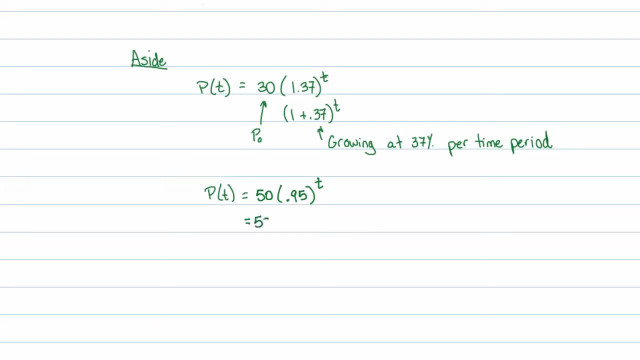 But you still can use it, because this is like 50 times 1.. 1 minus some number, And that number is .05.. What this is telling me? you can think of it in two different ways, actually. You can either say: this is telling me that every year that passes, or every week that passes. 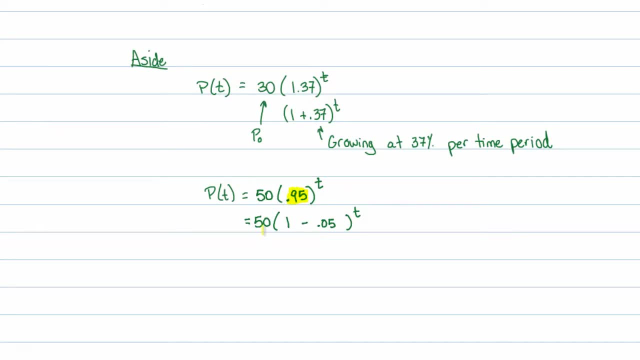 I retain 95% of my students. That's every week. Or you could say, conversely: every week that passes, I lose 5%, I lose 5%, I lose 5%. Same, I'm saying the same thing. 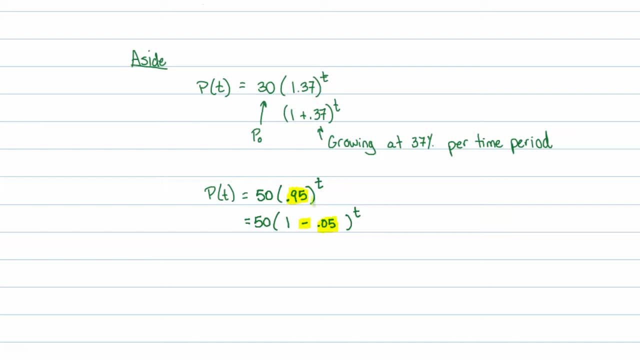 So either I keep 95% or I lose 5%. Glass is half full, half empty, whatever you want to use, And this is just saying I initially have 50 students And I lose 5% per week. Let's just pretend that's true. 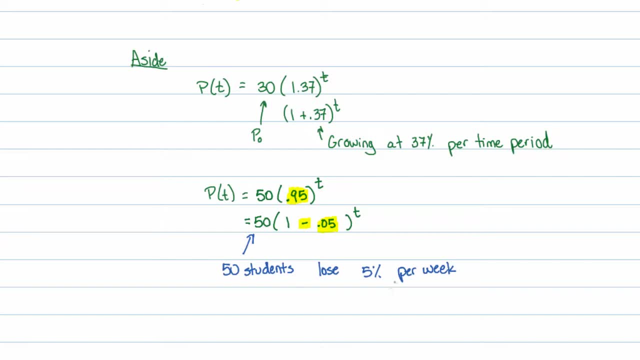 Okay, So now you can determine how many students are in my class after 15 weeks. This is just made up data, by the way, So let's get back to our problem now that I've kind of taken some time on this aside. 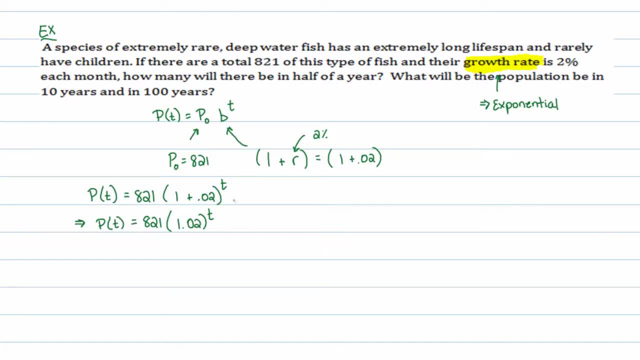 to do a little bit more here. So now, when you look at this problem, when anybody hands you an exponential function, you should always think, oh, there's some type of population of 821 objects growing at 2% a year, or whatever it is. 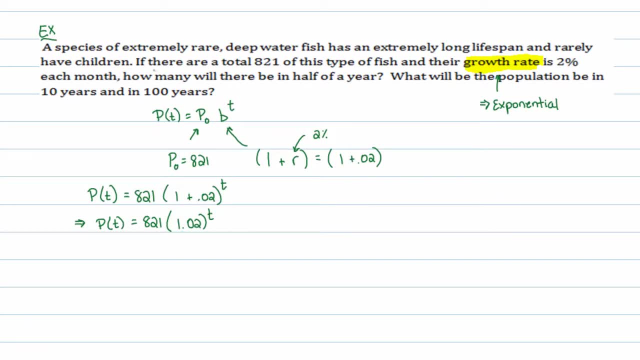 Okay, In this case, a month, 2% a month. How many will there be in half a year? Well, T is in terms of months, So I need to find out how many that are going to be there half a year. 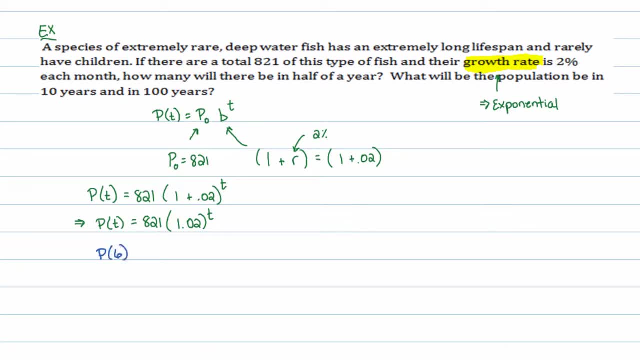 That's 6 months. So I want to know what P of 6 is. That's going to be 821 times 1.02 to the 6th power And, of course, something like this. I'd rather use a calculator. 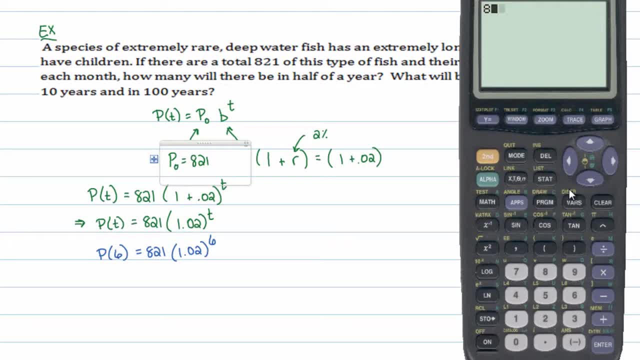 So I'll go ahead and open up this thing and put in 821 times 1.02, raised to, And I get 924.. And let's just round it down because technically it is a population of fish And so you can't have, you can't round it up. 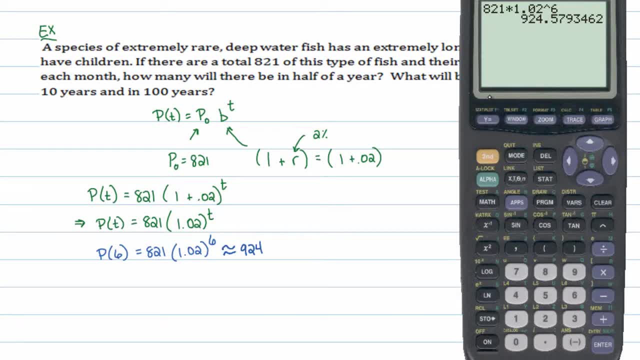 You have to round it down honestly, just to be realistic, You can't have .6 fish. Okay, So that would be roughly the population after 6 months, And And then the next two parts are: just how many do you have after 10 years and after 100 years? 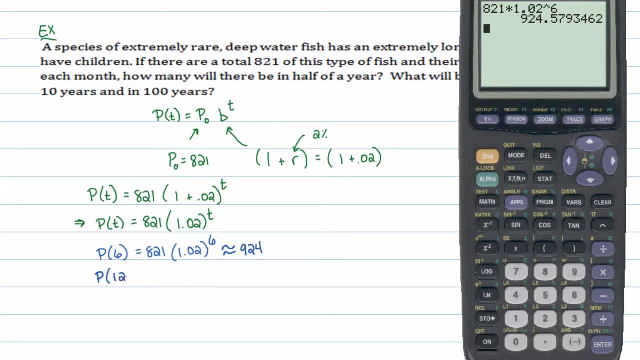 Well, 10 years is just 12 months per year times 10 years, which is going to be 120 months, And 100 years. 12 months per year times 100 years would be 1,200 months. I'll just plug in: 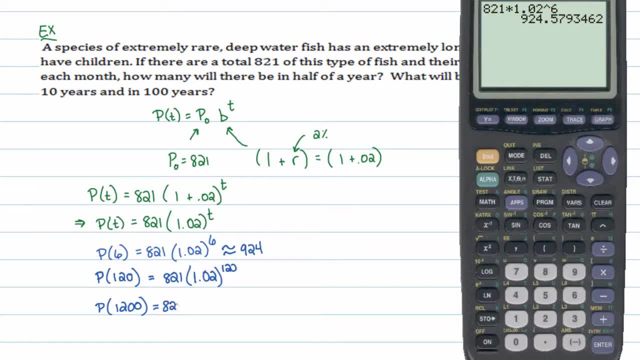 120 for the, The values of t in the function, and 1,200.. We'll see what we roughly get here. Should be somewhat of a slow growth, but who knows? So let's see. Second answer: bring back this. oops, I don't have any answer. shouldn't have done that one. 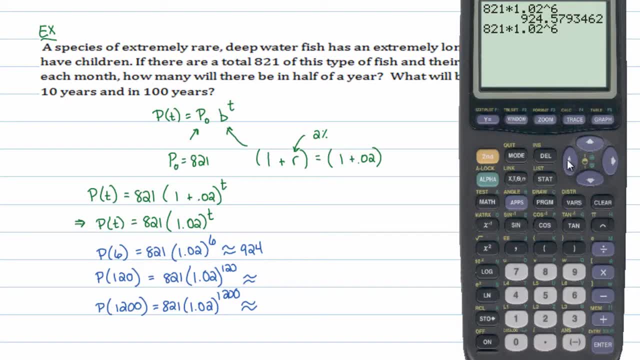 We'll do second entry That gets back our last entry And I'll just put in 120 instead of that sin. And I'll just put in 120 instead of that sin. And I'll just put in 120 instead of that sin. 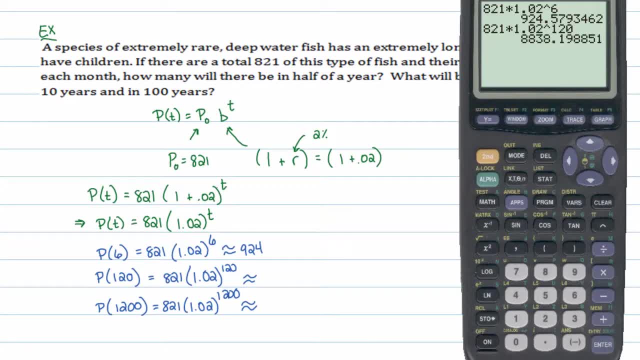 So that's six, 8,838.. And now again, second entry, to bring back your last answer, And I'll just put an extra zero on there And I get a huge population. This is 100 years later than the. it's crazy. 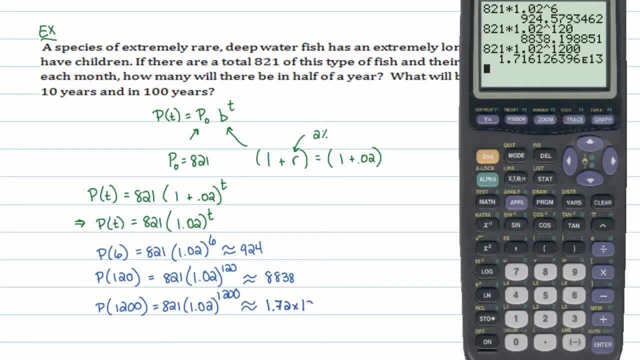 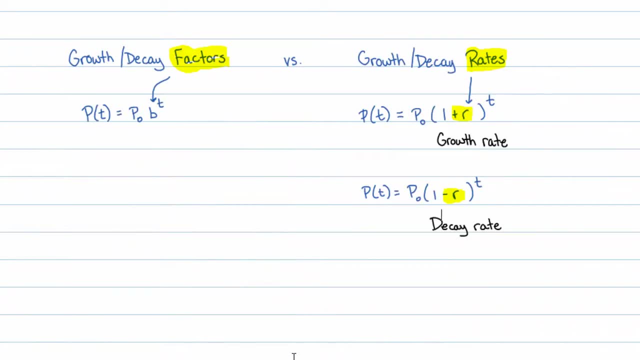 So it's one point. I'll just say: 72 times 10 to the 13th power, Quite a few fish. so again, I just want to bring it back to the two basic forms of an exponential function. either you're given a growth factor explicitly, like tripling and all that fun stuff, or a growth 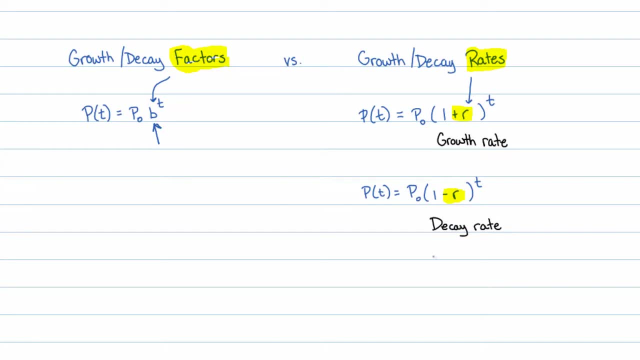 rate or a decay rate, and we've dealt with both of these. now I sincerely despise not going into why the growth rate formula is the way it is. some people just go: well, I'll just accept it. well, I'd rather show you why it is the way it is. so let's show you why that population function. 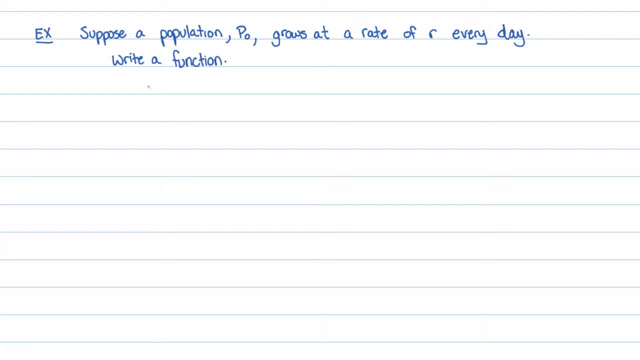 is the way it is when you're talking about growth or decay rates. so suppose I give you some initial population. it grows at a rate of r every day. let's go ahead and write a function. well, the best way to start if you don't have a population function, is to write a function. 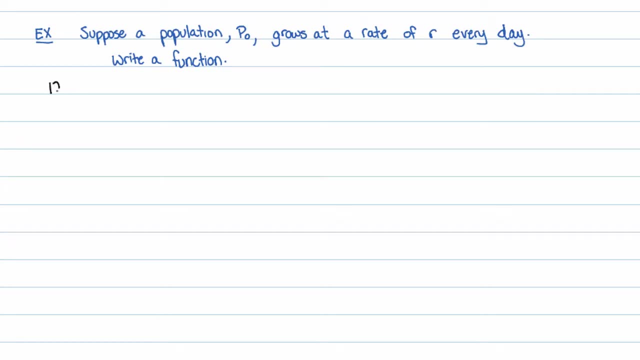 the best way to start if you don't have a population function is to write a function. don't know how to start. a problem is: think of money or something like that. if you had a hundred dollars and it grows at ten percent a year, that means next year you'll have how much? so if you 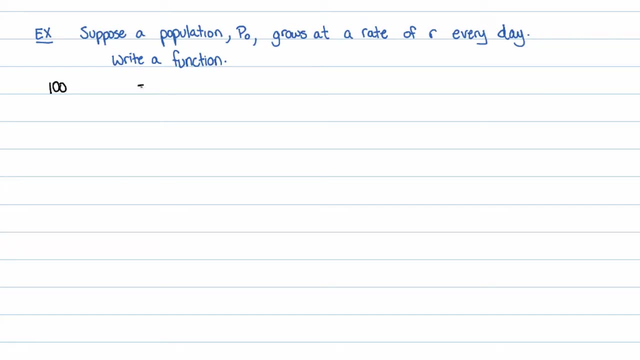 have a hundred dollars this year. it grows at ten percent a year. that means next year you'll have a hundred and ten dollars, right? how did you get that? I mean people just say: oh I, you know I get ten percent of all. I have students that say ten percent of a hundred gives me a hundred and ten. 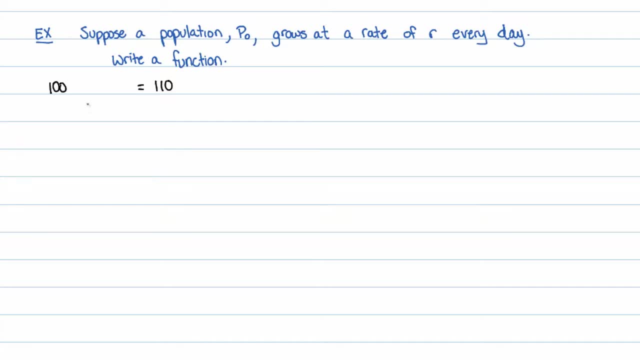 no, ten percent of a hundred is ten. you add that back to your regular initial hundred dollars. so you started with a hundred dollars and what you did is you added ten percent of that one hundred dollars to get 110. well, that's essentially saying this: 100 plus 0.1 times 100. that 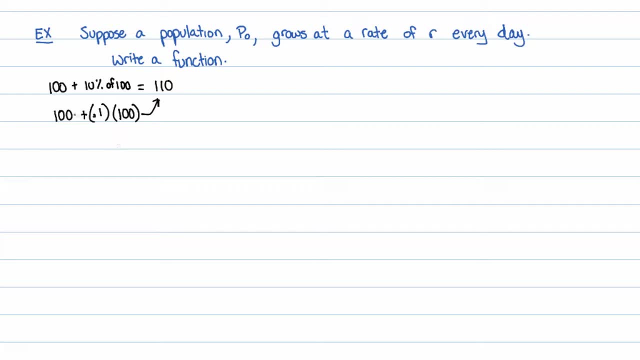 gave me that 110, didn't it? what you should notice about both these numbers is these 100s, is that they can factor out the. both these terms here have a hundred in it, so I can factor that out front what I'm left with. well, if I factor a, 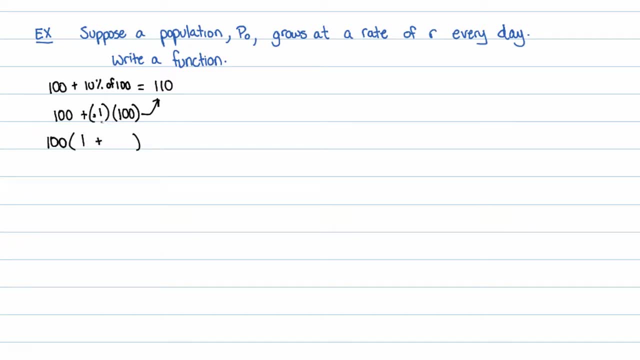 hundred off this first term, I'm left with the one. if I factor a hundred off the second term, I'm left with a point one, but it should still equal 110. now I'll show you where I'm going here. let's go ahead and build a table for this situation. 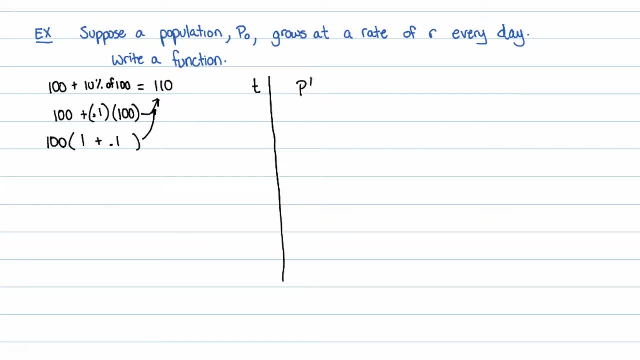 so this is the thing about this history: when you go back, one like you'll see here, you'll see an. I can't compare to anything you played against up until ten percent, jump in, or you know if I were having a good day playing my media, そう, just after theредition or two up with my ability. hybridization doesn't. 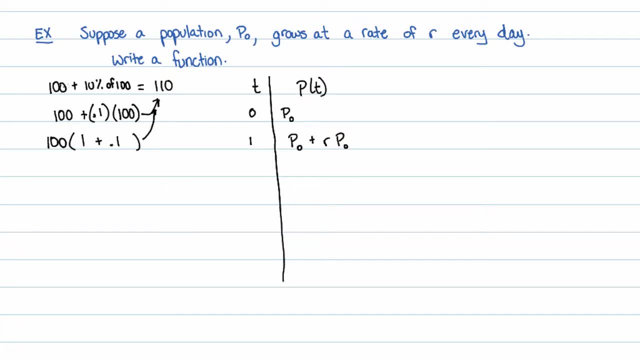 mean that was good or not good. it only just gives me an idea of that, my ability to'm not automatically gonna color change every time we start here in thousands in a set up order why we started 100 P if we had 10 percent, that number two justrance dollars by zero, so at times zero, two times us 0 and and our population at that time? so 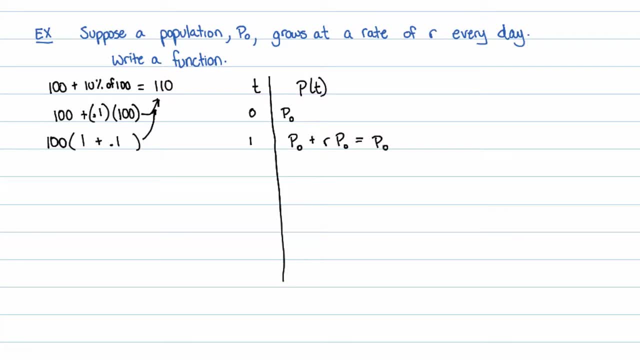 at these two terms. they have a p naught in common, so I'll factor that out. I'm left with one plus r. okay, so that's what the population is after one day. by the way- notice, the power on this is one two days later. well, the population is initially going to be what it was yesterday. this population, 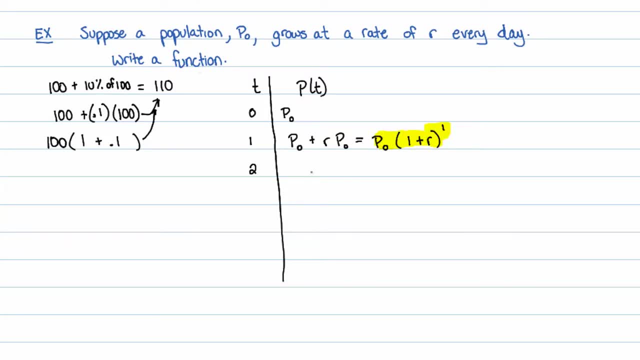 right here, so let me write that down. so at the start of day two, here's our population: p naught times one plus r. but it's going to grow at this rate of that population from yesterday. so in other words, we have yesterday's population plus we tack on a certain percentage of yesterday's. 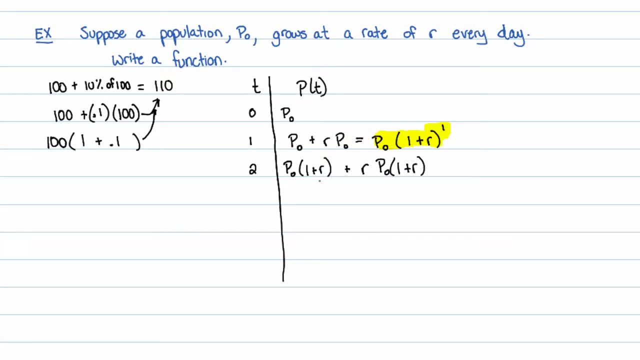 population. now, if you look at this expression, you- both these terms- have p naught in common, so I'll factor that out, and a one plus r in common, so I'll factor that out front as well. when I do that, the first term is left with a one. the second term 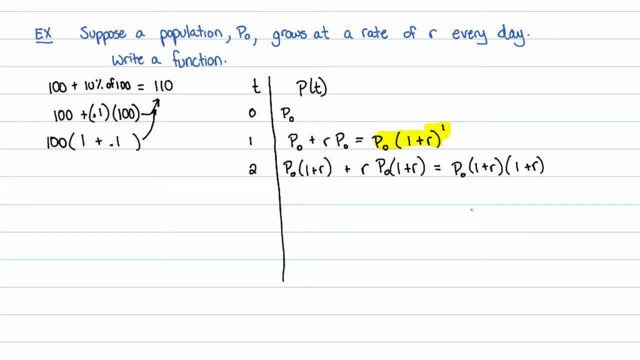 is left with an r and all of a sudden you see that's going to be p naught times one plus r squared. now you could probably see the pattern already. right, you can see the pattern on the left where I simply draw something. I drew it so on the right side. 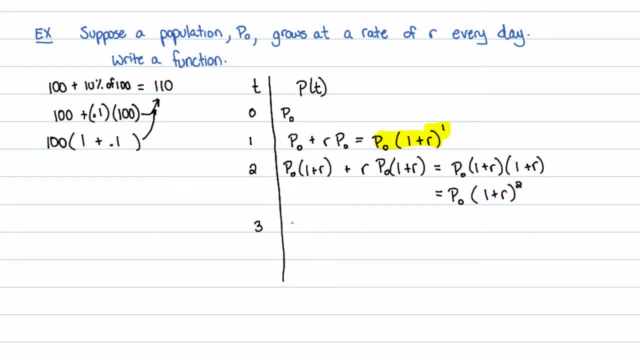 here and ant грue and then here I'll actually keep the fr classical assassins. so it should be better with an a plus R for the first time. ok, day 1 it's p knot times 1 plus R. to the first day two, it's people at times 1 plus our. to the 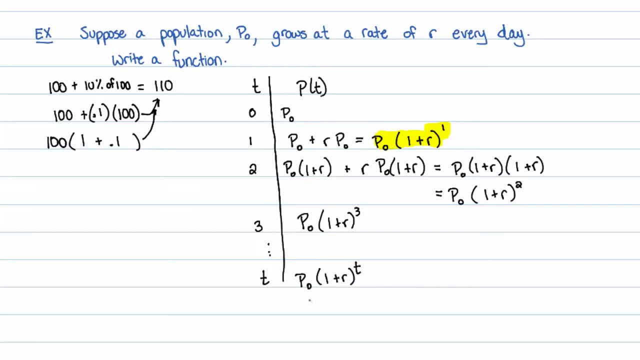 second, obviously day 3, your probably the population will probably P, not times 1, plus R to the third, and so on and so forth, until you get today- whatever you want, let's say day T- that the population on day t is going to be p, naught times 1 plus r to the t power. 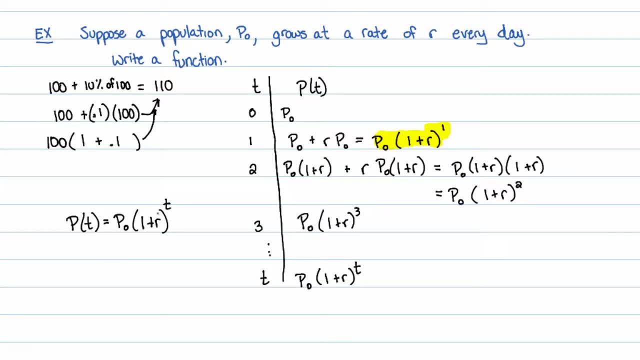 which is exactly what we said, is the exponential function when you're given a growth rate. So that's why the growth rate function is the way it is, because you're constantly just tacking on 1 plus r. You're multiplying last year's population, or last day's population, by 1 plus r. 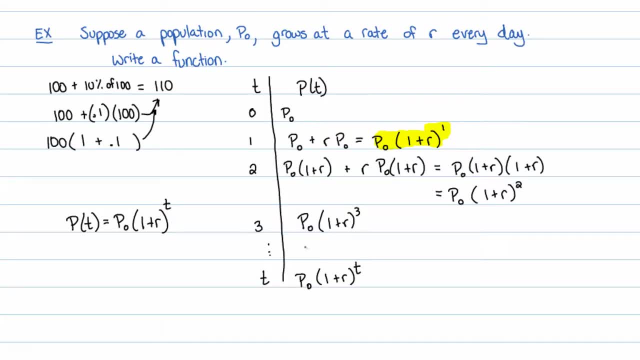 And I understand that a lot of students don't like these extended diatribes about how to derive these things, but the fact is, if you don't know why something is true, then don't bother learning it right. It's useless to learn something. 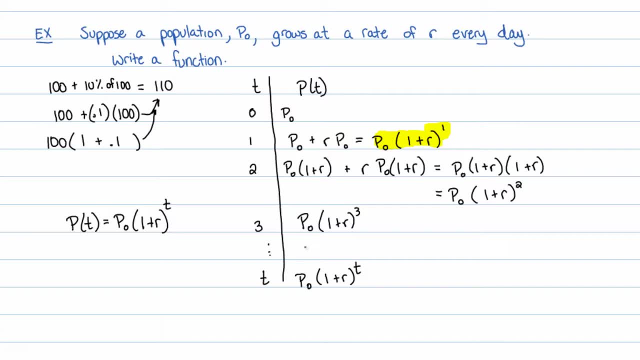 You're not really learning, you're just mimicking. you're just being a parrot if all you do is go around and just swallow what somebody tells you without thinking about it. So please bend your mind around these. Let's take another example. Inflation is suspected to be about 6% over the next 9 months. That means after 9 months, the value of something that was $1 today will be $1.06 in 9 months. Right now, a certain car costs $18,000, so let's pretend. 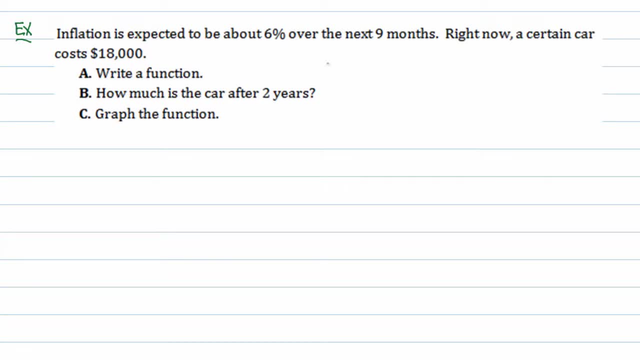 So write a function for this. And to write a function for this, first of all they've given me a growth rate. So this rate, right Right here, tells me it's growing by 6% every 9 months. That's exponential growth, right there. 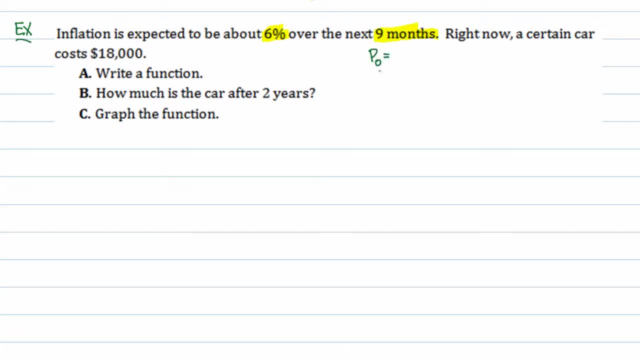 And in fact they've told me the initial value, the initial population value for the car is $18,000.. And I know that B, which is the growth factor, can be written as 1 plus because we're growing in price .06.. 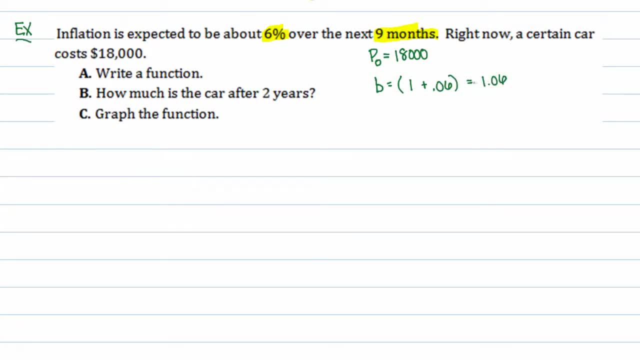 So that's 1.06.. And technically that's actually not true. true, because I told you that we're growing at this rate once every 9 months. So it's actually going to be 1.06 to the one-ninth power. 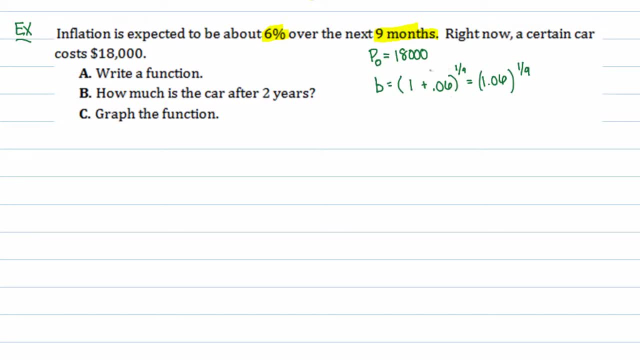 Remember how this works is that if you do this every single month, if it's growing by 6% per month, then you don't have to worry about it. It's 1. It grows by this factor once every one month. 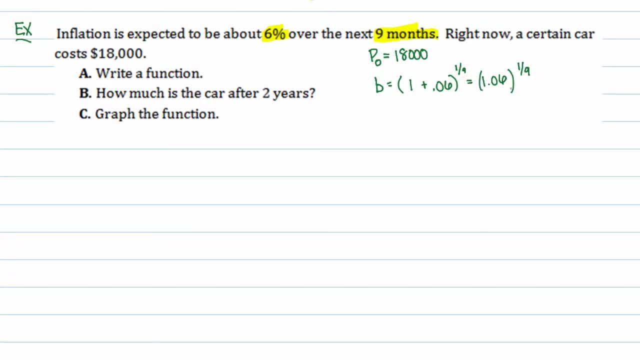 But it only grows by this factor once every 9 months. So you have to have that one-ninth power on there. So let's go ahead and write our function. Our function is just going to be P of T, and you don't have to use P all the time, but I tend to like to. equals 18,000 times the base raised to the T power. 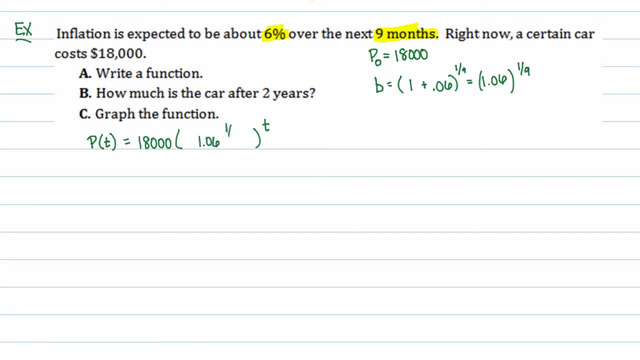 And the base we said is 1.06 to the one-ninth power. I also told you in the last problem I don't like to write it like this. I like to write it like 18,000 raised or times 1.06 raised to the T over 9 power. 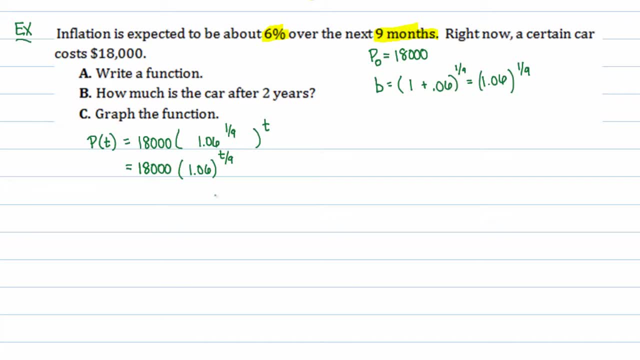 It doesn't really matter, They're both the same thing, It's just I don't prefer to write it the first way. How much is the car worth after 2 years? So 2 years, we're talking months, though T is in months. 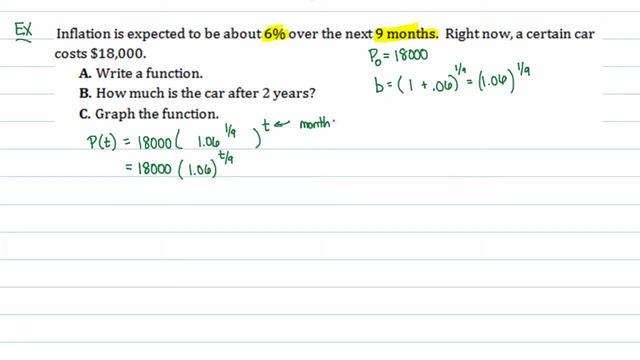 Be very aware of that. So when they ask you- and this is a very common thing in life- that you, just you always mix units in life, just how it is. So when they ask you how much the car is worth after 2 years, convert that to months. 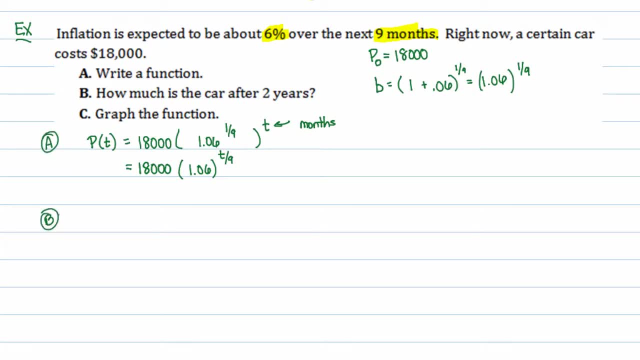 So part that was part A, Part B, we're going to say what is P of 24, because that's 24 months. Well, let's see 18,000 times 1.06 raised to the 24.. 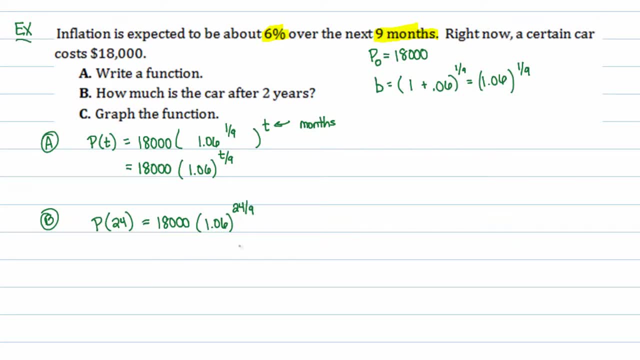 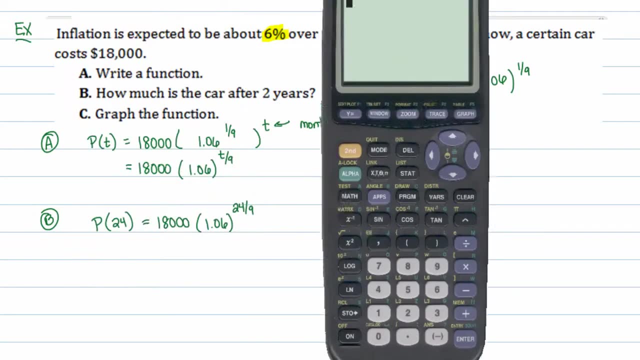 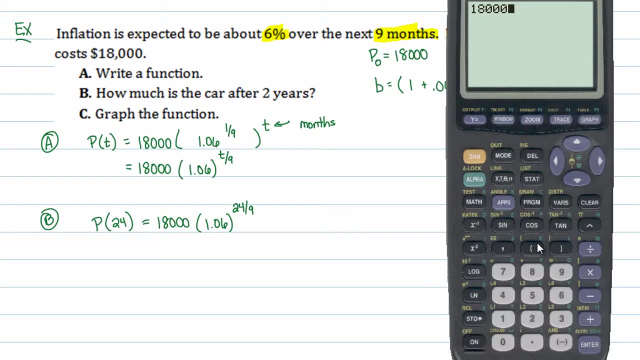 No use in reducing that fraction, because the fact is I'm going to be grabbing a calculator no matter what, So I don't even bother reducing the fraction. Reducing fractions is only useful if you are not going to, if you're not allowed to grab a calculator. 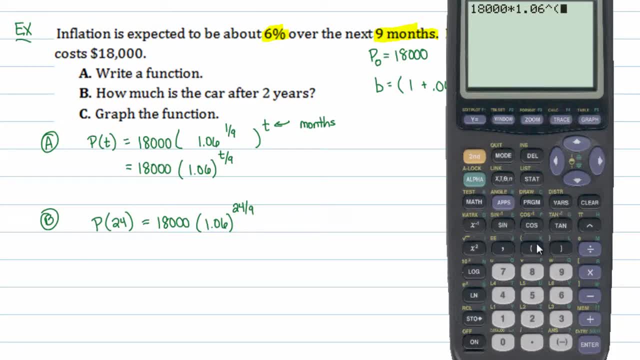 And we'll raise this to the and remember there's math in my exponents, so I have to start with a parenthesis there: 24 ninths, 21,025 dollars and 91 cents, Roughly equals to. it's been approximated as 21,025 dollars and 91 cents. 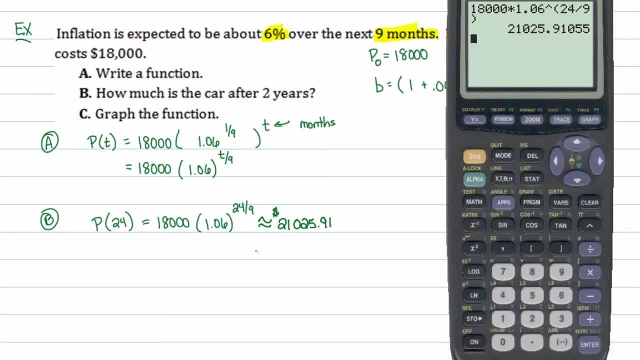 So if you don't buy it today, well, you can buy that car in a couple years. it's just going to cost you an extra 3 grand. Last part of this is asking me to graph This function, And really, if you're going to graph this function, the best way to graph it honestly is to use this version right here. 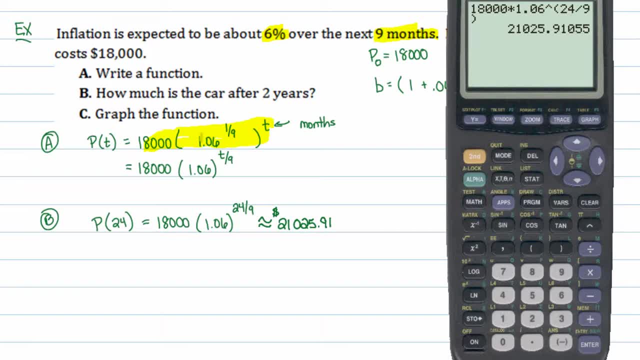 In the long run. that's how you're going to graph these. So when we talk about exponential graphs in future lectures, it's going to involve that first form, because it really does make it nice When you're doing that. But one thing I'll do here is I'll convert 1.06 to the 1 ninth power. 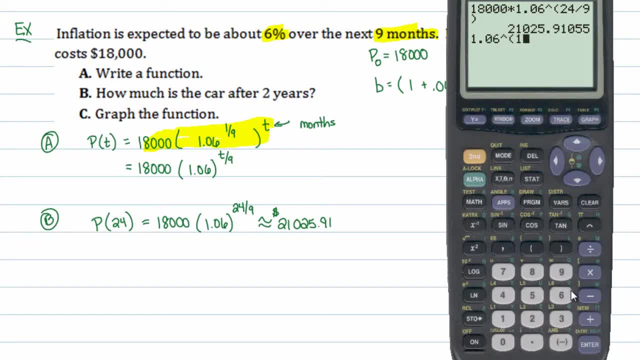 I'll just find out what that actually is. Let's see here, 1.06 to the 1 ninth is a number a little greater than 1.. So really, I'm just going to delve into this a little bit further. 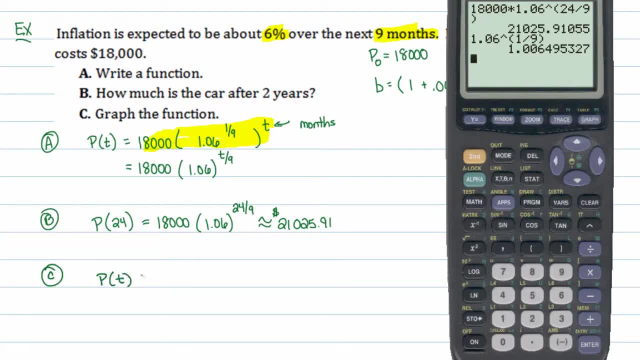 So for part C, I'm going to first say that P of T is really not equal to now. It's roughly equal to 18,000 times 1.00649.. I'll put on a few more decimals: 5,, 3,, 2,, 7.. 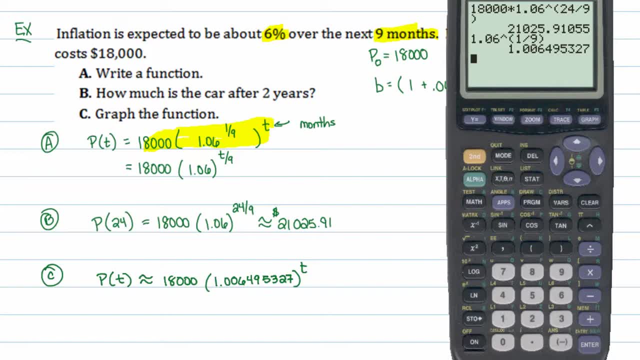 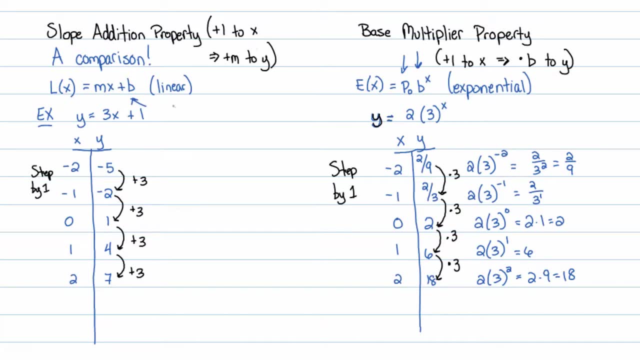 To the T power And remember what I mentioned in the conceptual lecture. In the conceptual lecture I was comparing linear functions and exponential functions. I said Exponential functions have a really unique property, Just like the linear functions do Linear functions: when you increase the value of x by 1, the outputs get added to by the slope. 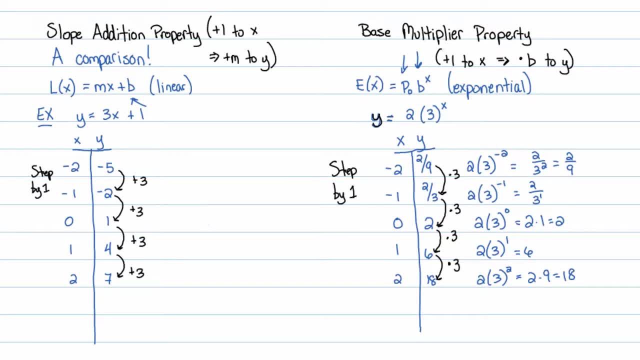 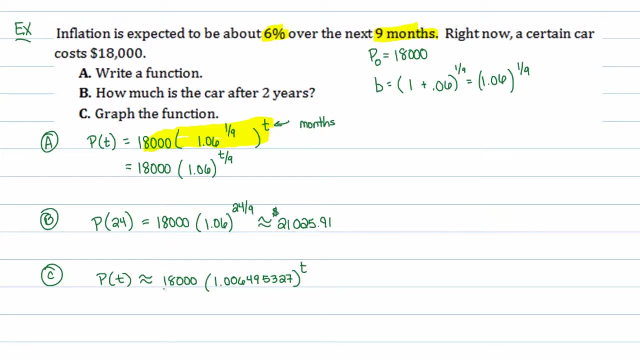 That's why we call it the slope addition property Exponential functions. when you step by 1 in the x direction, you're multiplying the output by the base. So, coming back to this example, I know that initially the cost is 18,000. 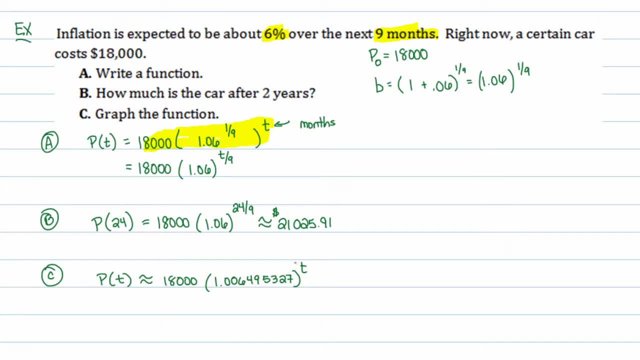 And every single month that passes, I'm multiplying that value by 1.00649 and some change Right, Since that number is slightly larger than 1, that means that this product, 18,000 times that number, is going to be slightly larger than 18,000.. 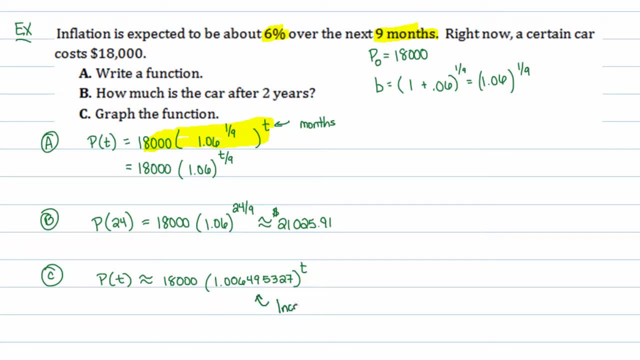 This right here means it's an increasing graph, And that's just because the product between 18,000 and that number, once we start using it, is going to grow 18,000.. Now, to be honest with you, if you were asked to graph this by hand, you would just plot some points. 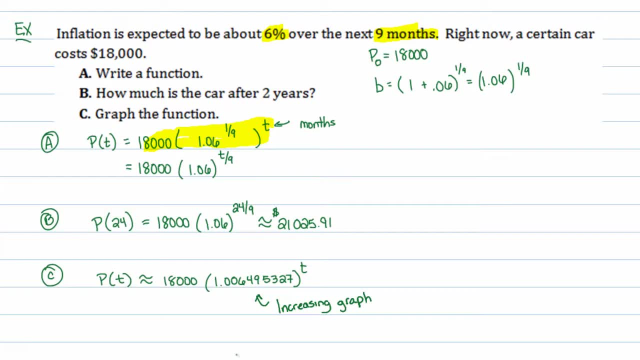 Plug in: T equals 0,, which you already know is going to be 18,000.. And then T equals, let's say, 5 or 9 or whatever you want to plug in. Okay, But what I'm going to do is just show you on a graphing calculator what it comes out to be. 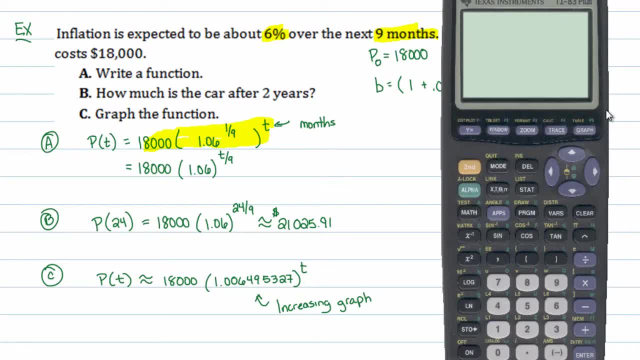 And for those who have graphing calculators, this is a good point to pay attention. Remember all the graphing functions are accessed via the top five buttons. I'll hit Y equals here, clear out any old graphs, And I'll type in 18,000 times and I'll start a parenthesis and I'll say 1.06.. 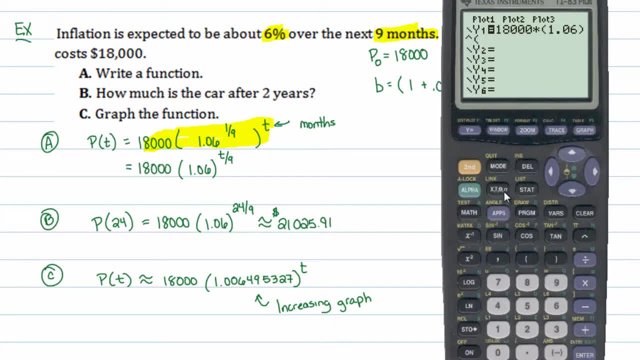 End that parenthesis And raise it to parenthesis X over 9.. Notice how I'm mixing these three different versions of my function. It's just this second version is easier to type in And I didn't choose this version I wrote down here in part C because that's only an approximated version. 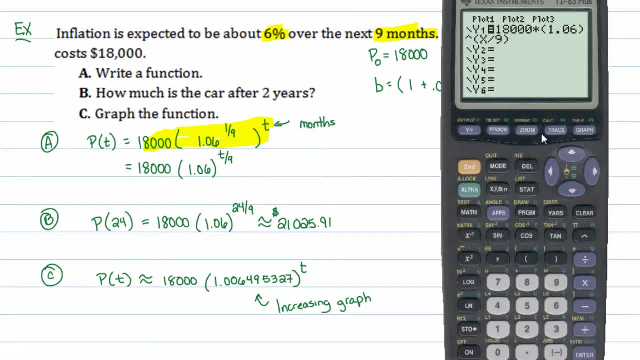 I want an exact version, So I'm just doing it this way. Now, if you hit graph, you're likely not going to get very much on your window. The reason why is your window's not set up. You have to show a value of a car. 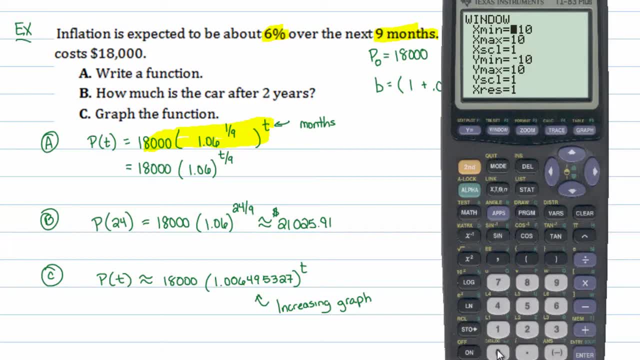 So what you want to do is you want to adjust your window and say, well, let's say starting this year. So remember, our inputs are the number of years that have passed or number of months that have passed. And well, let's go out to a two-year period. 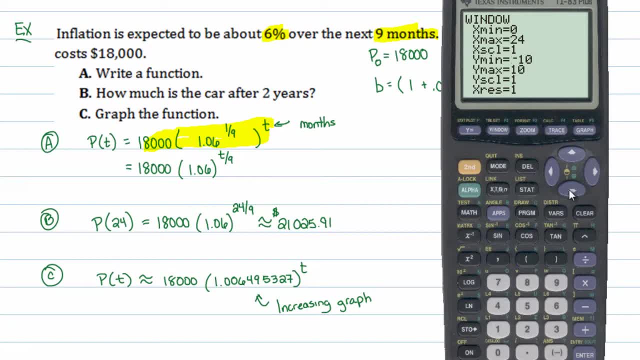 Oh wait, but two years is 24 months. There we go. Now the minimum Y value: The Y values are the outputs and these are the values of the car, And the lowest value of the car is 18,000.. 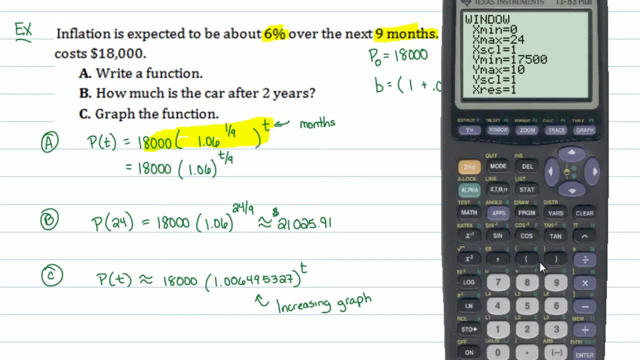 So maybe I'll start my outputs at, let's say, 17,500.. And the maximum I'm going to say- well, I know the value after two years is 21,000.. So I'll say 22,000.. 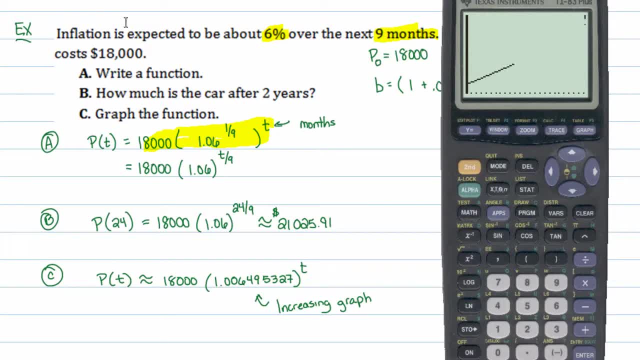 If I hit graph now, you'll see. there it is. Here's my exponential function. It looks like a line, doesn't it? It's not a line. It's growing ever so slowly. So you just have to trust me that that is not a line. 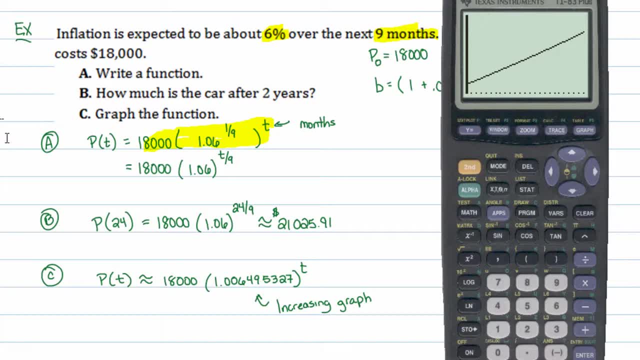 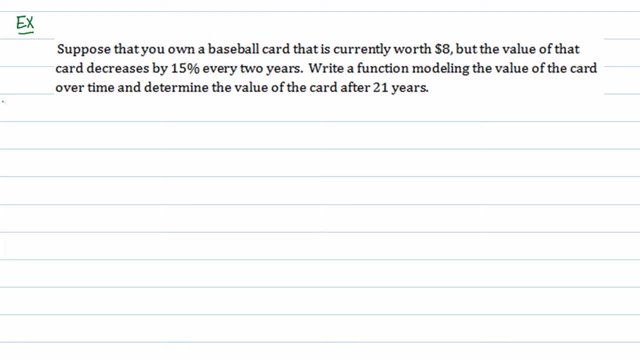 It's actually just growing really slowly, But it keeps growing. It keeps growing faster and faster, just not as fast as most exponential functions that you see. Now, this is kind of an apropos example for something I was just doing this evening. 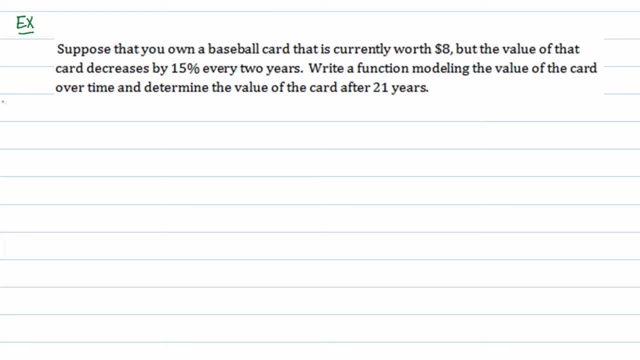 I have a friend that collects comic books, and he came over and asked me to help him value some of his comic books, And so this is all about collecting objects and their values after a certain number of years, And if you know that the value of an object is increasing every year, well then you'd like to keep it. 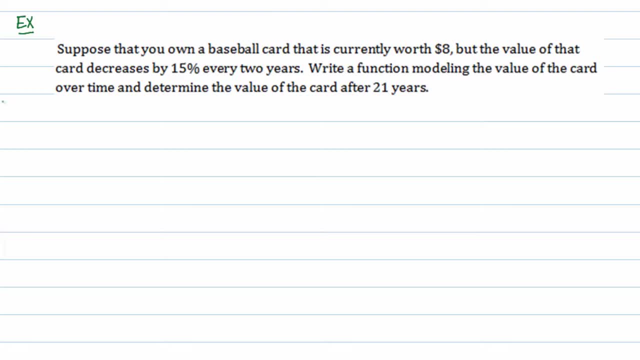 But if you know it's decreasing every year, it's probably good to get rid of it. So let's suppose you own a baseball card that's currently worth $8, but the value of that card decreases by 15% every two years. 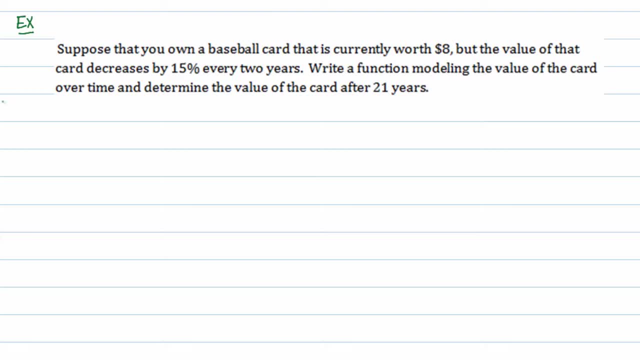 Write a function modeling the value of the card over time, And then you do this And determine the value of the card after 21 years. Okay, Well, I know the initial population. Well, first of all, I know it's exponential because it's decreasing by 15% every two years. 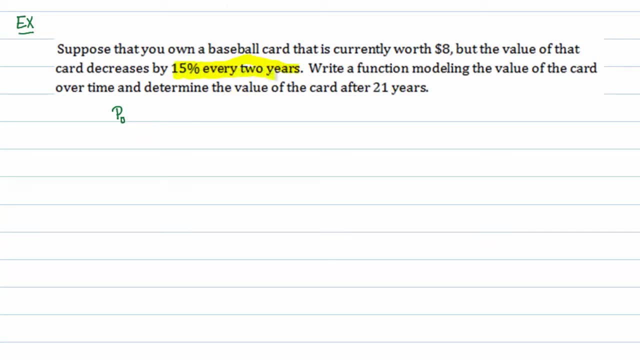 This phrase right here tells me this is an exponential function, Not linear, not quadratic, but exponential. And I know the initial population is 8.. That's the initial value And I happen to know that the value of b is going to be something like: well, let's see, it's decreasing. 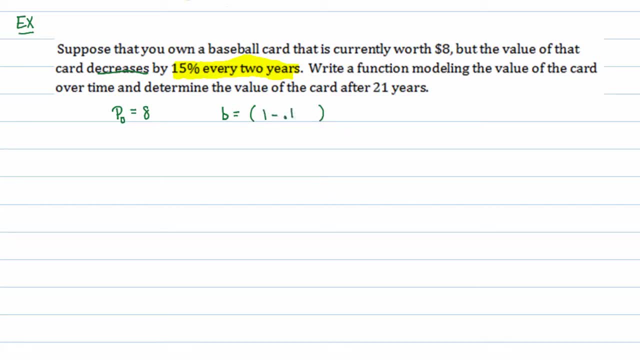 So it's going to be 1 minus 15%: 0.15.. Now, it's not just this, because it drops by 15% not once every one year, but once every two years. So there is the decay, The decay factor. 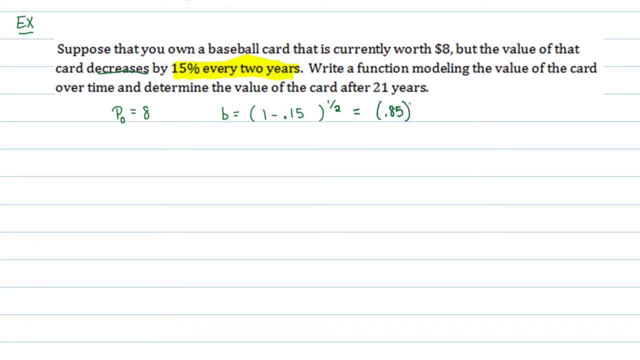 And actually you can kind of clean this up and write this as 0.85 to the one-half power. So there are a couple of ways you can think about it. You're losing 15% every two years, Or you're retaining or keeping 85% of the card's value every two years. 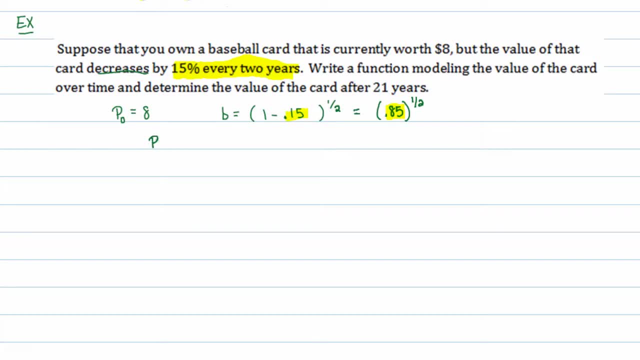 Whichever way, It's the same thing, So let's go ahead and write the function itself. The population of the value of the card after two years is equal to 8 times 0.85 to the one-half, not to the one-half to the t over 2 power. 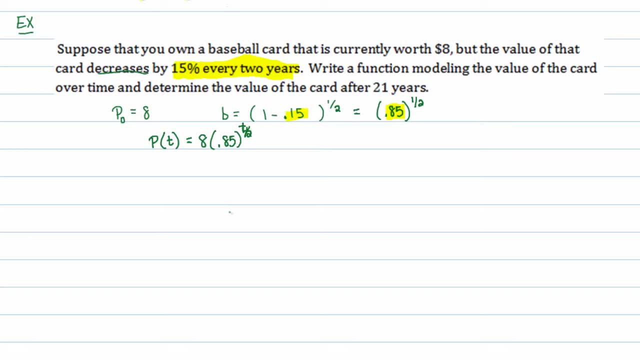 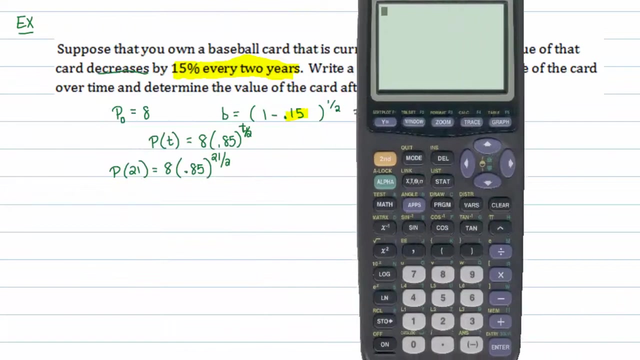 Okay, All right. So let's go ahead and now find the value of the card after 21 years. Well, it just means: p of 21 equals 8 times 0.85.. So the value of the card after 21 years is equal to 8 times 0.85, to the 21-halves power. 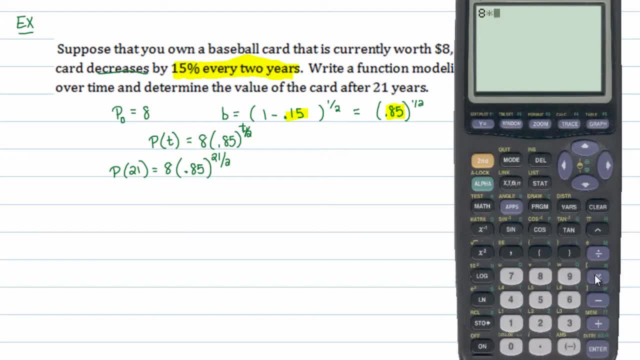 And again you just open up a handy-dandy graphing calculator or any type of calculator. Scientific works just as well. 8 times 0.85, raised to the 21-halves power, Here we go. 8 times 0.85.. 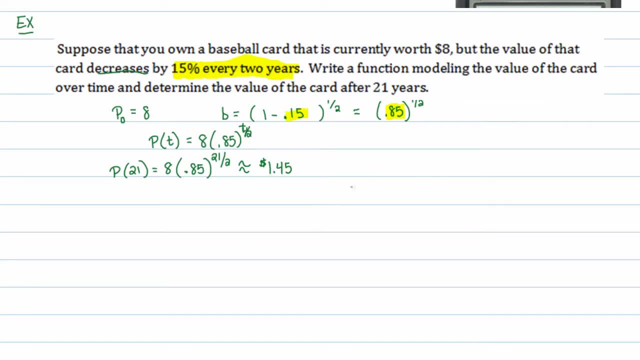 Not worth a lot actually, after 21 years, By the way. take an economics class or something like that, and you'll find out that it's actually worth a lot less, because the fact is dollars are, dollars inflates, or the dollar loses its spending value as time goes on. 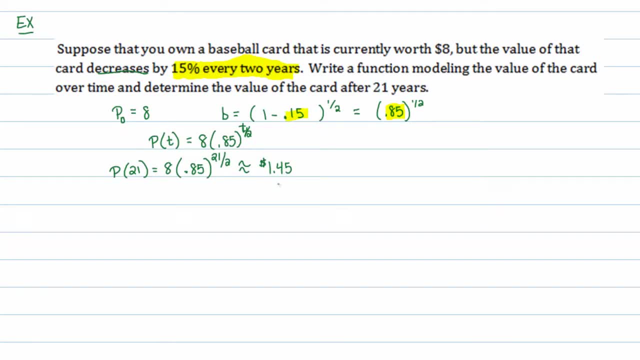 So that baseball card that was worth $8 today. if it's still worth, if that $1.45 is in today's dollars, it's actually worth much less in future dollars. So that's kind of an interesting little note. One thing you want, though, is you want to make sure that you buy the baseball, if you're a card collector or something like that. 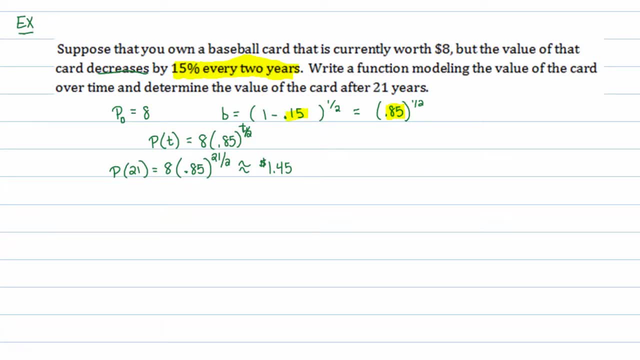 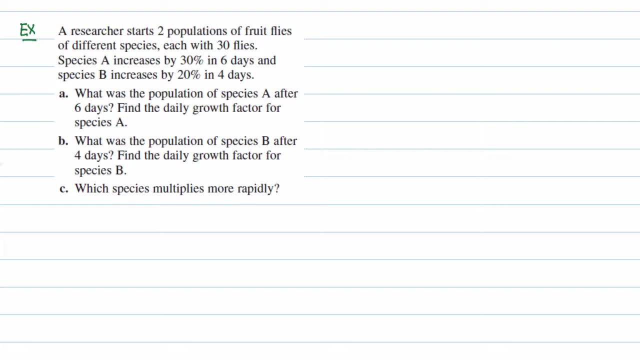 buy something that you know people are going to want. That's all I've got to say after sifting through about 400 comics tonight. Okay, Let's suppose a researcher starts two populations of fruit flies of different sizes. Let's say we have two populations of fruit flies of different species, each with 30 flies. 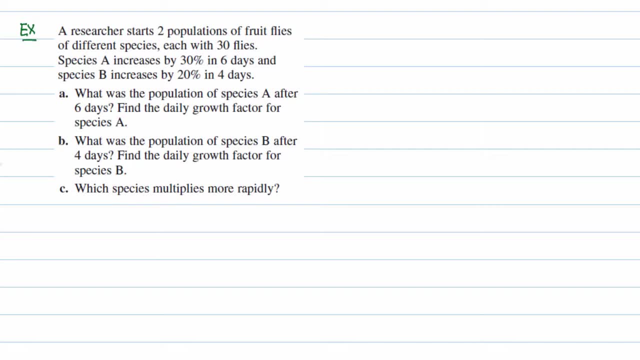 So we have two different populations going on. Species A increases by 30% in six days and species B increases by 20% in four days. What is the population of species A after six days? Find a daily growth factor for species A. 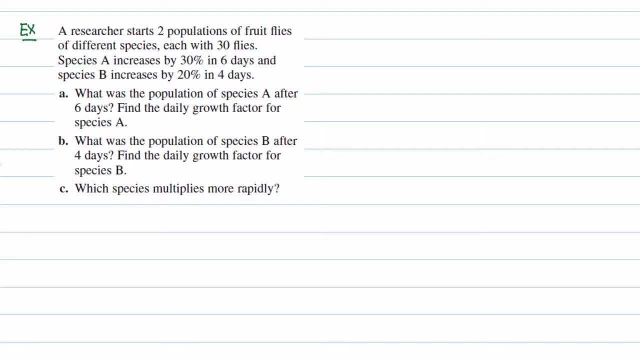 And then what's the population for species B And find the daily growth factor for species B And which species grows more rapidly. Okay, So there's a lot of. it seems like there's a lot to this problem, but it's actually not too bad. 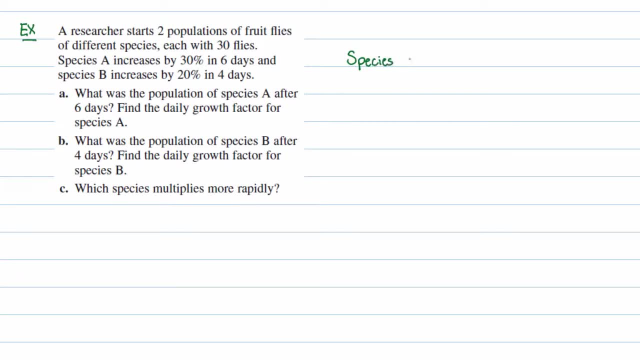 We have just two situations, two functions, one for species A and one for species B And for species A. for both of them, actually, the initial population is 30 fruit flies, So let me just start with that. Now I have to multiply them by a base. 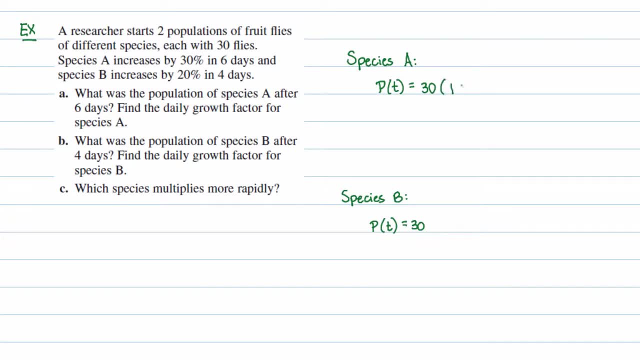 Species A is increasing by 30%, So that means one plus .30.. Every six days, So T over six. And species B increases by 20%, So one plus .20. And again that's every Four days. Well, you know, I hate having it written like that. 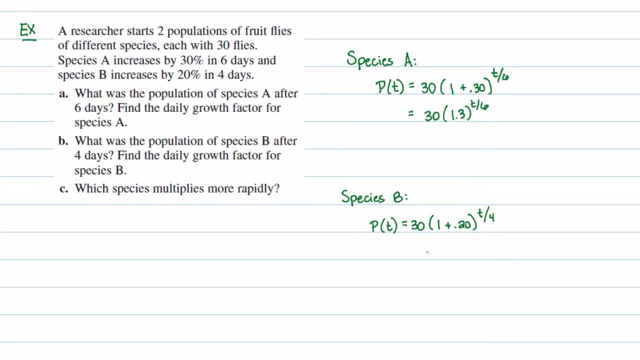 I'll just write it as 1.3 to the T over six, And this will be 30 times 1.2 to the T over four. The question really is which one's growing more rapidly? Well, let's see. 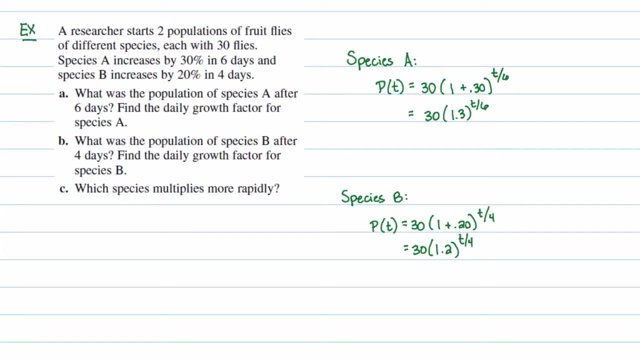 Species A. Honestly, I don't like how this question's asked. It's a great question, Don't get me wrong, But I don't like the fact that they're having you well, actually. no, I think it's okay. 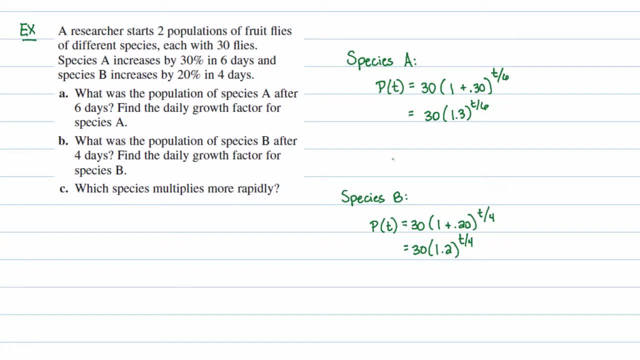 Let's find the population species A after six days. Now I'm reading it. It actually does make sense, So let's go ahead and do it. Population after six days here is going to be 30 times 1.3 to six over six power. 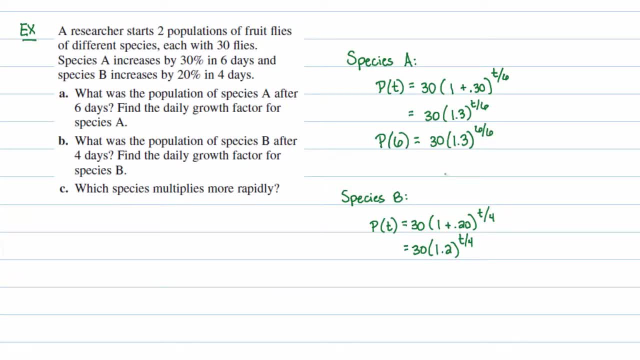 Or in other words, the first power. Now I'm just going to, rather than bringing up the calculator, I'm just going to use the calculator in my hand right now And that comes out to about, not to about. it comes out to exactly 39.. 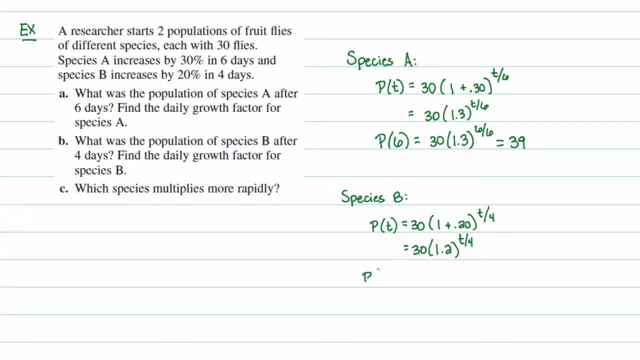 And down here, population B after four days is going to be, let's see, 30 times 1.2 to the four over four power. In other words, to the first power That is actually going to be 36.. 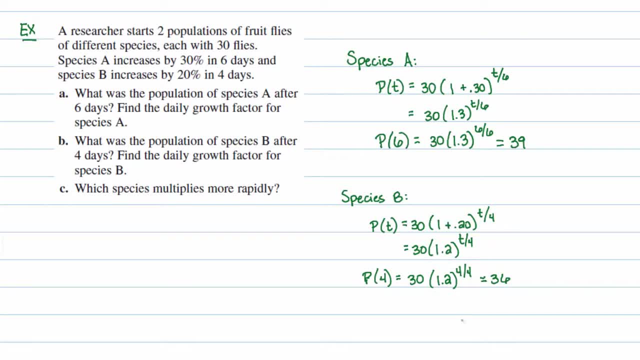 Exactly So. let's see, Looks like species A grew by more, But you're talking two totally different periods of time. For species A, that was six days that it got to grow to 39. Species B only had four days And it grew to 36.. 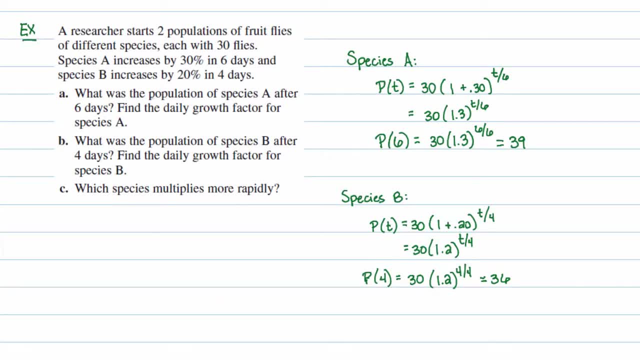 That's a pretty healthy improvement. Now, before I answer the secondary parts of parts A and B. So we already answered this was 39. And this right here was 36.. I need to mention something that I sort of well I'll blame myself. 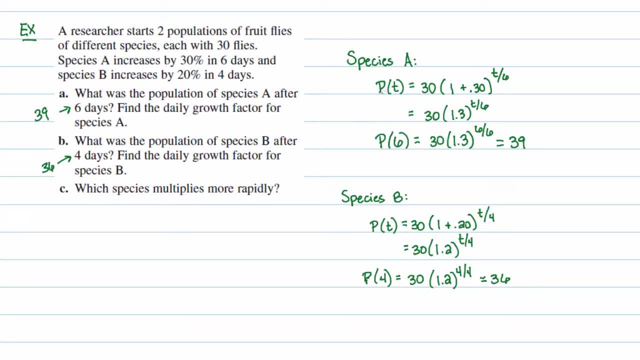 It's sort of messed up here Is that I shouldn't label both these P. They're two totally different functions. I should call this P sub A, So it distinguishes itself as a function from the other function. This should be P sub B. 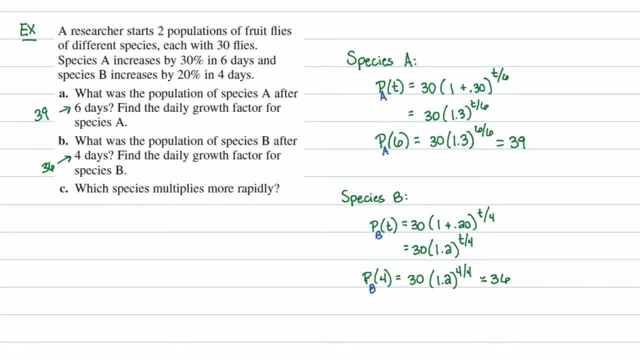 That's a little no-no. I really shouldn't do that. You shouldn't label two functions with the same letters if they mean completely different things. Okay, All right, So find the daily growth factor for each of these. Now, remember the growth factor is not 1.3 for this part A. 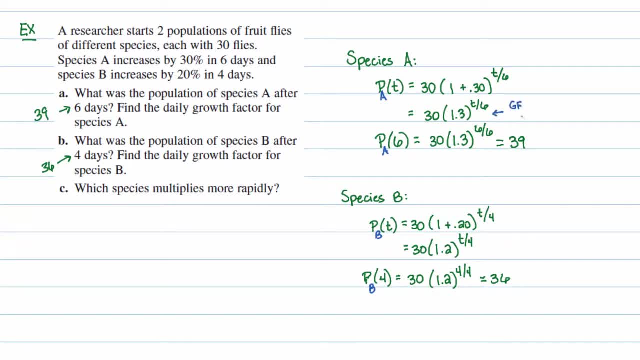 It's actually going to be. so the growth factor here growth factor- It's going to be 1.3.. Whoops, 1.3, raised to the 1 sixth power, And the growth factor is going to be 1.3.. 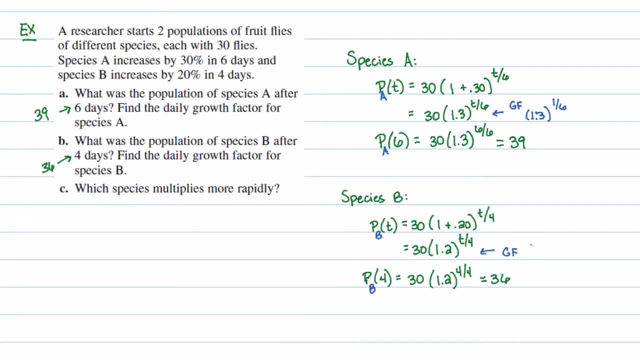 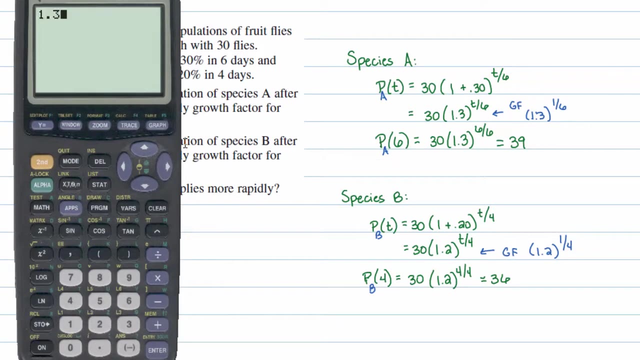 And the growth factor for species B is going to be 1.2 to the 1 fourth power. So this is where you grab a calculator. Well, maybe I will bring one up here just to illustrate this Type in 1.3.. 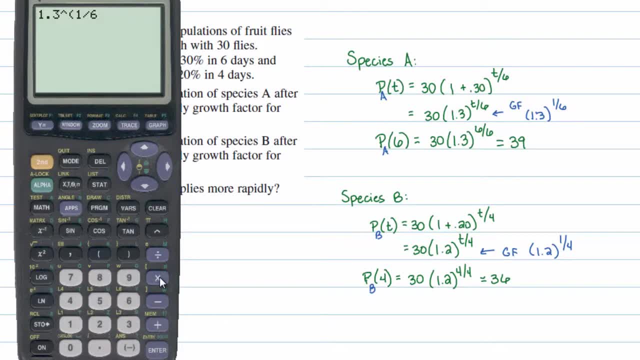 You raise that to the parenthesis. 1 sixth power, I get 1.044.. 1.04.. 1.04. 1.05.. That's for species A, So 1.045.. Roughly That's the growth factor. 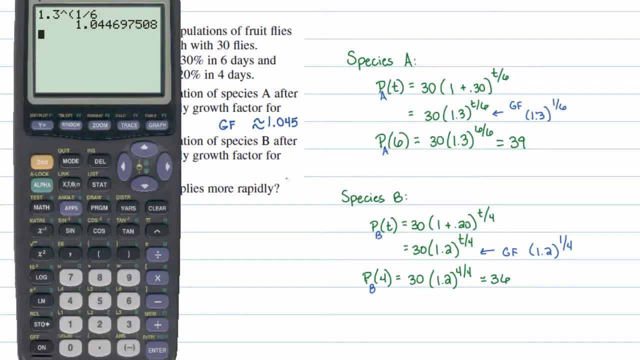 Now let's see for species B. We had 1.2.. Oops, Typing it there And I'm mean to be typing it up here. 1.2 raised to the again, start a parenthesis And it will be the 1 fourth power. 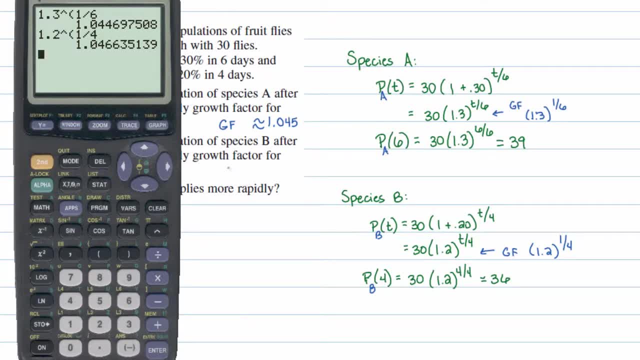 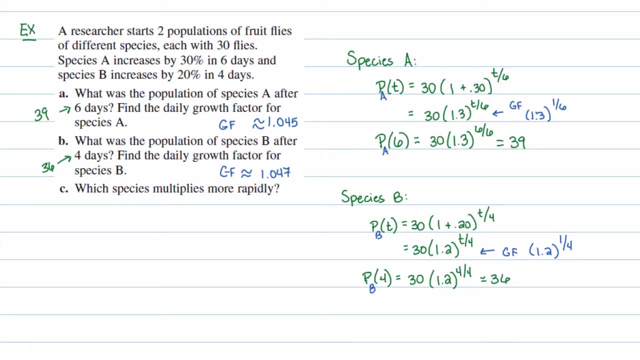 It's 1.47, 1.047.. Now compare these two growth factors. Which one is a larger growth factor? Well, this one right here is which means that species B is actually growing more rapidly, So on a daily basis growing more rapidly. 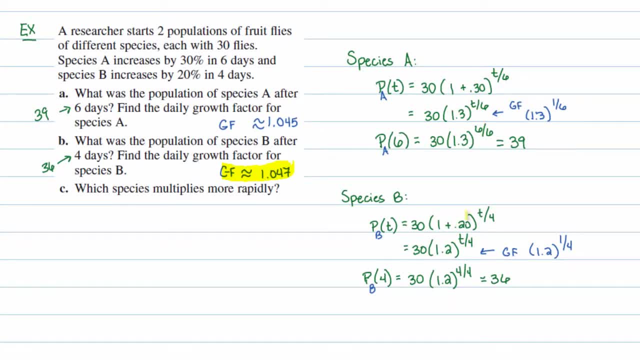 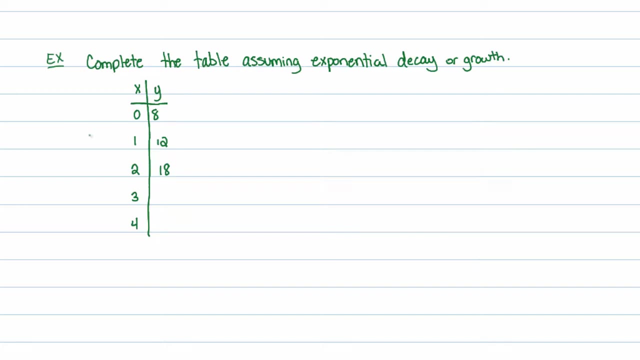 So, given time, that species will just blow up faster than species A, All right, not so bad. Now, I was going to save this last example, these last two examples, for a different lecture, but I really don't want to waste a different lecture on just two examples. 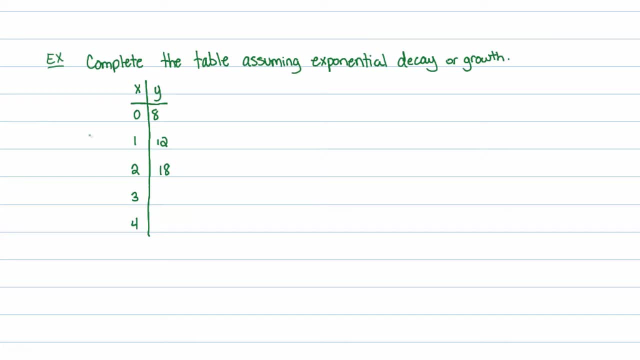 It essentially is bridging the idea between the two: The base multiplier property that we talked about a few moments ago, and using the base multiplier property to create a table. Now, remember, with an exponential function which we're going to assume this table represents. 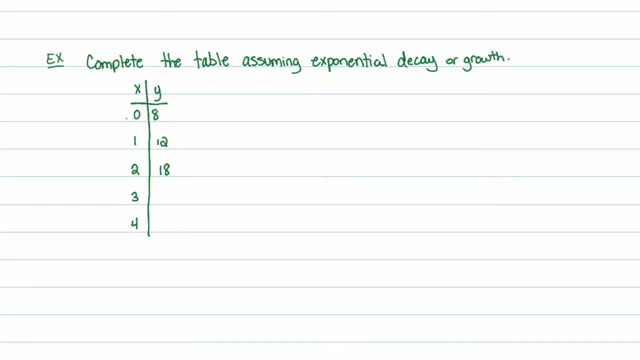 each time you take a step in the x direction of one unit, you are multiplying the outputs by the same number of units, By some number, but we don't know what. The question is: what did I multiply 8 by to get to 12?? 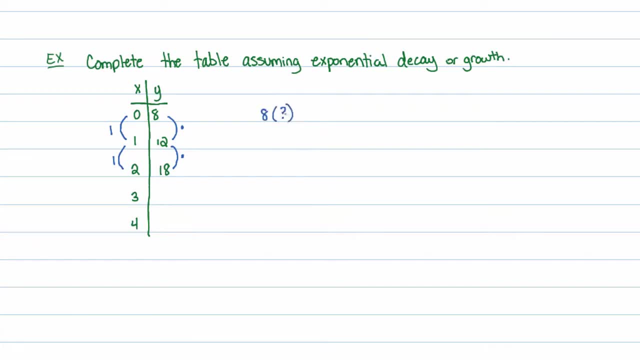 So, 8 times what value is equal to 12?? And the answer is well, divide both sides by 8, you'll find that the value is going to be nope, not 4,, 3 halves, Okay, so this tells me that to get, 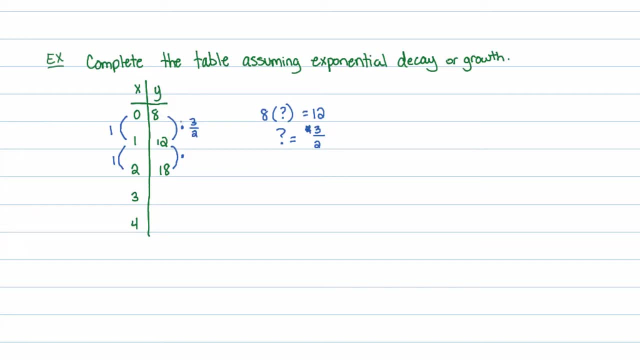 from 8 to 12,. I will multiply by 3 halves. Check it out: 8 times 3 is 24,. divided by 2 is 12.. Let's see if that holds for 12 to 18.. 12 times 3,, that's 36, divided by 2 is 18.. 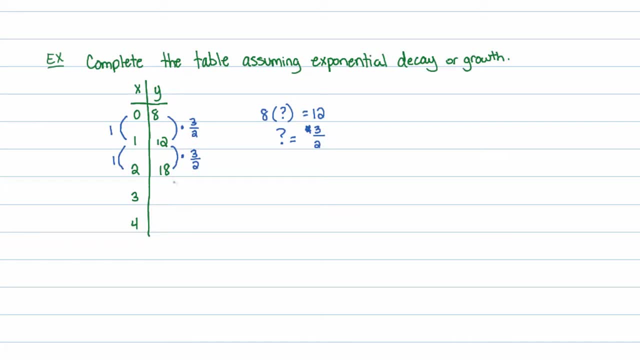 So I guess I did multiply by 3 halves to get to 18.. So let's find these two last missing values here. I'll write them in black. when we find them, I know I'm going to have to multiply that last, since I'm stepping back a little bit. 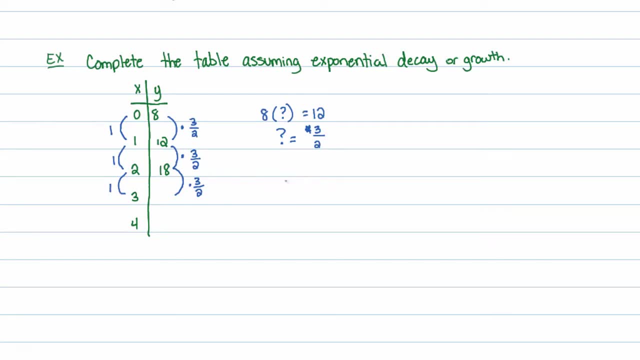 stepping by 1 on the x value. I'll multiply the y value, the last y value, by 3 halves. So 18 times 3 halves. Well, 2 goes into 18. 9 times 9 times 3 is 27,. 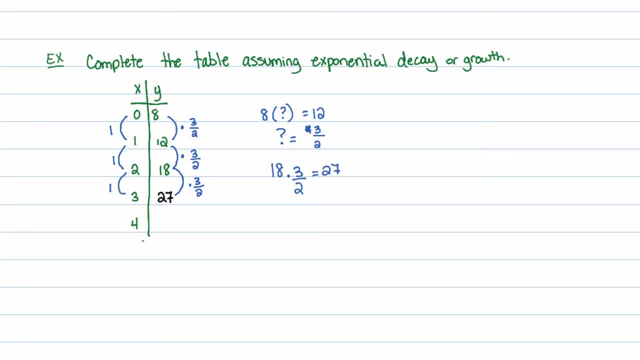 so this should be 27.. That's the unknown there. And again, stepping from 3 to 4 means that I'm going to multiply the output by again 3 halves Using the base. this was the base multiplier property. 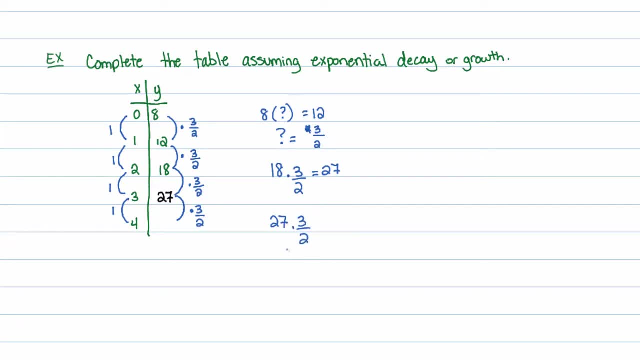 So the output before was 27,. I'm multiplying by 3 halves, And this one is not so nice, It's just 81 halves. there's not much really that you could say or do about that. You can't simplify it. 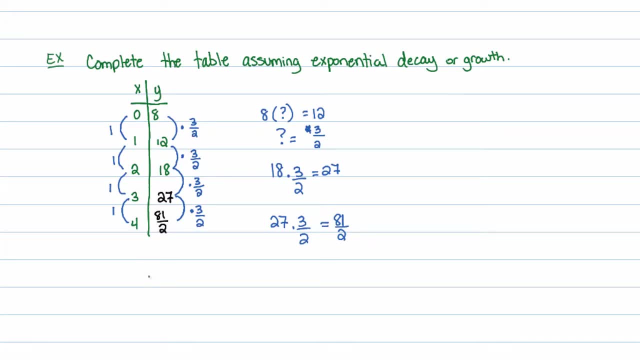 So it's just 81 halves. So there we go: 81 halves. Base multiplier property is pretty neat. it helps you really fill in the table very quickly. great interpretation that, oh, every year that passes we multiply by three halves- very neat. now let's suppose this was example a, so i don't have to rewrite the 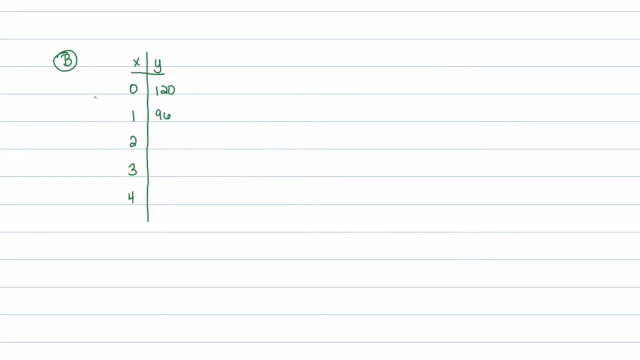 entire instruction here. so let's do this again with another table. in this table we again assume that it describes exponential growth or decay. okay, and i know that if i take a step of one in the x direction then i must have multiplied. if it's an exponential growth or decay problem, i must have multiplied. 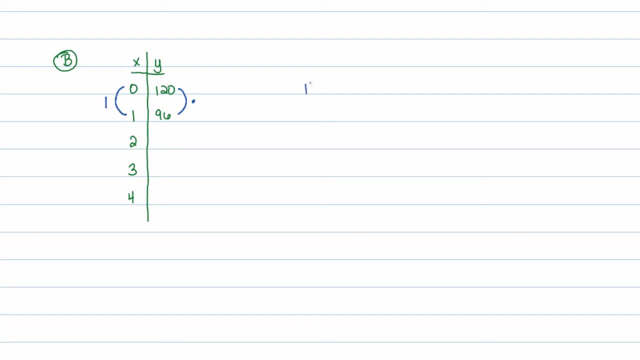 the output by some constant. so what do i? multiply 120 by to become 96, divide both sides by 120- oops, that's a question mark- equals 96 over 120, and those both. that fraction reduces down to four fifths after you do a little. 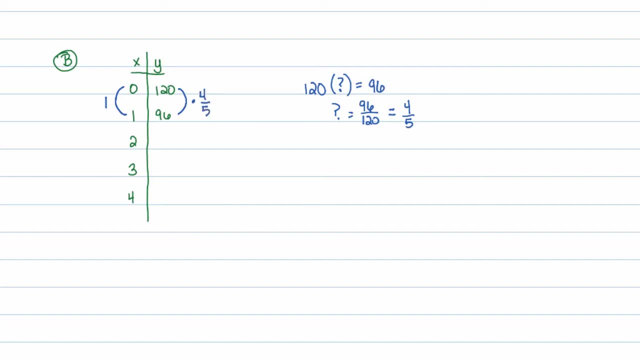 bit more of work there, so i know that i should be multiplying by four fifths. that's actually decay factor because it's a number less than one. the population is actually dropping and you can actually see it here: goes from 120 to 96, when i